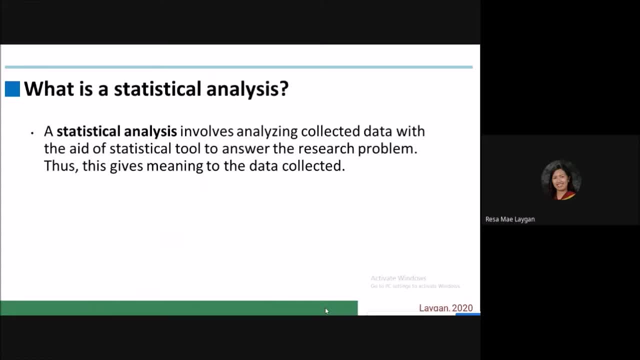 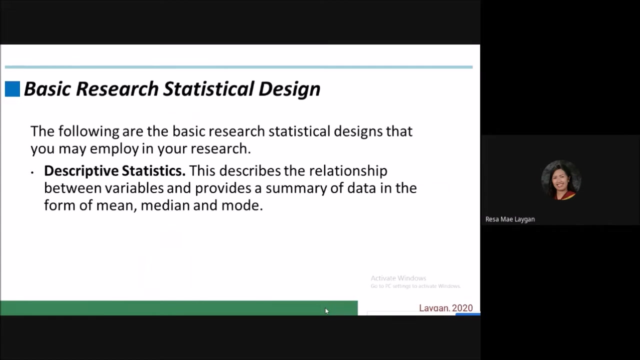 based on the data you have collected And based on each statement of the problem of your research study. So here are the following basic research statistical designs that you may employ in your research. We have the descriptive statistics, and actually this is common as it describes the relationship between the variables. 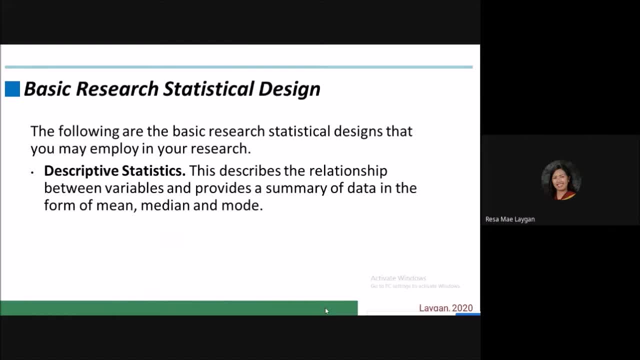 and it provides a summary of data in the form of mean, median and mode, and also you can describe the data in that under descriptive statistics, with the use of percentage frequency distribution. another is we have the inferential statistics. so on this, the data are analyzed from a sample to make inferences in the larger. 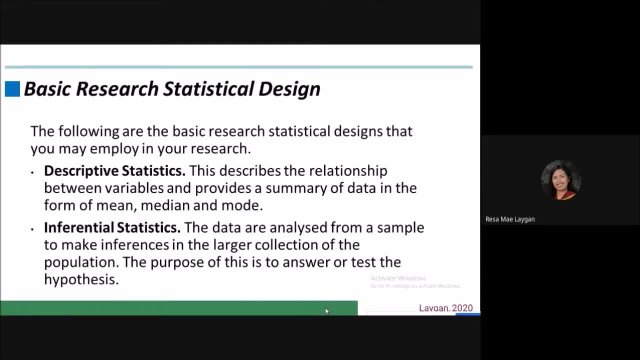 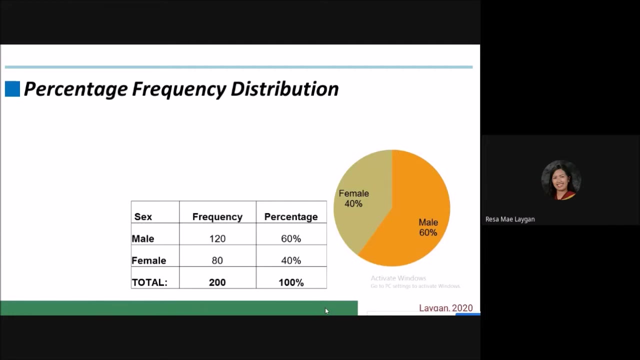 collection of the population. the purpose of the purpose of this is to answer or test the hypothesis. if your research attempts to test the hypothesis, you may use inferential statistic design. so here we are have the percentage frequency distribution. this is under the descriptive statistics, because you only summarize here the frequency and percentage of the data, particularly the categorical data. 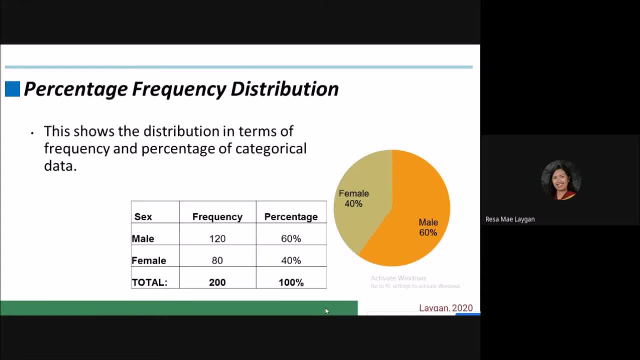 because when we say categorical data, these are the data that you categorize, this according to their criterion or according to their characteristics, for example sex. so we categorize sex into two: we have the male and female. so here, based in our data collected, we have 120 male respondents. 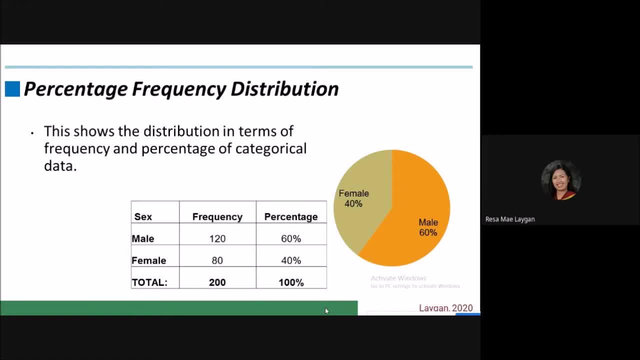 or 60 of the total respondents, and we have 80 female respondents, or 40 percent of the total respondents. so actually, um the frequency or percentage frequency distribution can be commonly done in charge or table, as you can see on this two figure, so you can choose the pie chart in order to 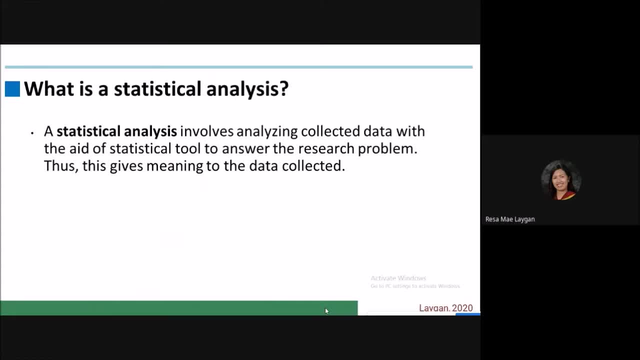 based on the data you have collected. Making statistical analysis is exactly the same, and the standard of Willingness will be based on each statement of the problem of your research study. So here are the following basic research statistical designs that you may employ in your research. 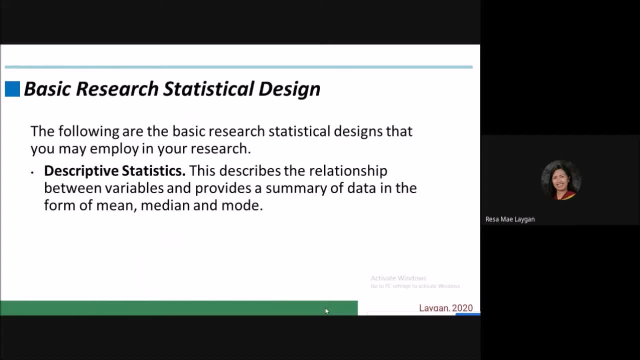 We have the descriptive statistics and actually this is common as it describes the relationship between the variables and it provides a summary of data in the form of mean, median and mode, and also you can describe the data in that under descriptive statistics, with the use of percentage frequency distribution. another is we have the inferential. 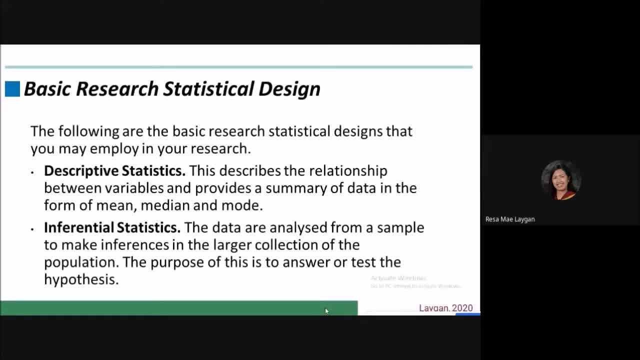 statistics. so on this, the data are analyzed from a sample to make inferences in the larger collection of the population. the purpose of the purpose of this is to answer or test the hypothesis. if your research attempts to test the hypothesis, you may use inferential statistic design. so here we are. 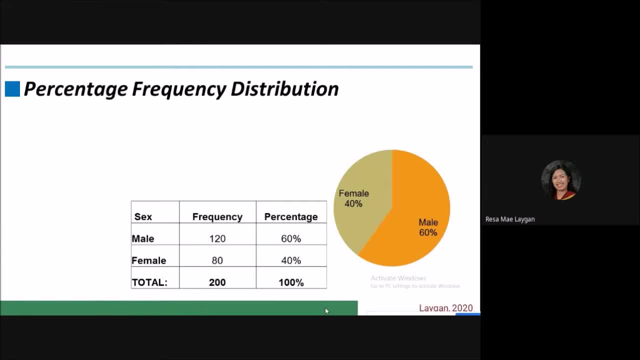 have the percentage frequency distribution. this is under the descriptive statistics, because you only summarize here the frequency and percentage of the data, particularly the categorical data, because when we say categorical data, these are the data that you categorize, this according to their criterion or according to their characteristics, for example sex. 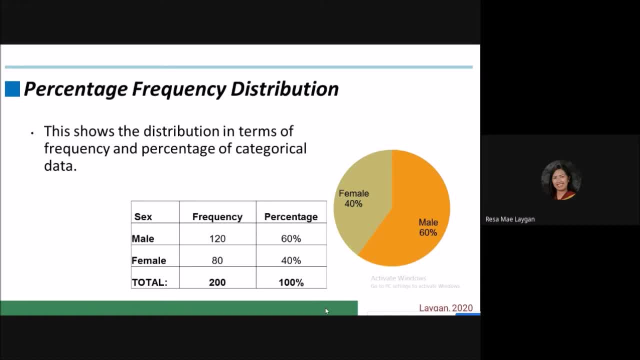 so we categorize sex into two. we have the male and female. so here, based in our data collected, we have 120 male respondents, or 60 percent of the respondents, and we have 80 female respondents, or 40 percent of the total respondents. so actually the frequency. 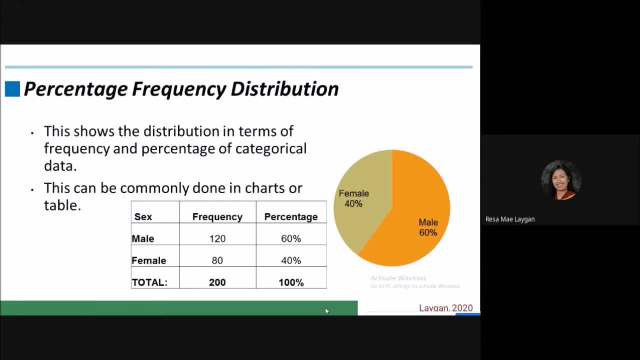 percentage frequency distribution can be commonly done in charge or table, as you can see on this two figure. so you can choose the pie chart in order to see the figure about the portion of each categorical data, or you can use the table to summarize the frequency and the percentage distribution of each. 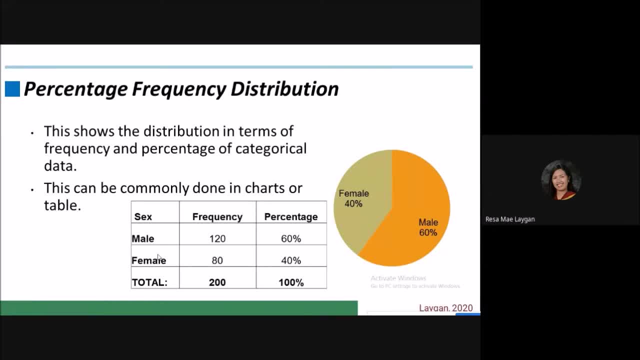 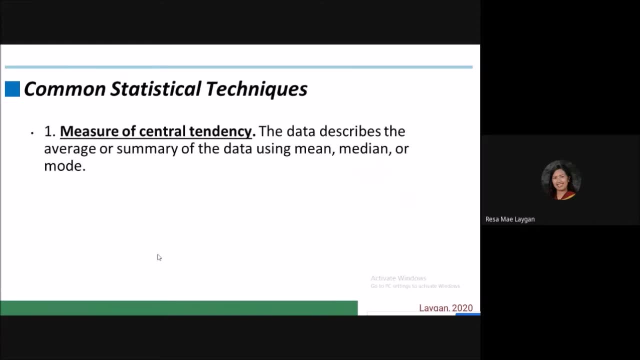 category called data. so we have also common statistical techniques here and we have the measure of central tendency. so in the measure of central tendency the data describes the average of the data using mean, median or mode. so these are familiar. so here you have to attest the center or the average. it can be through the mean, no, or the average or the. 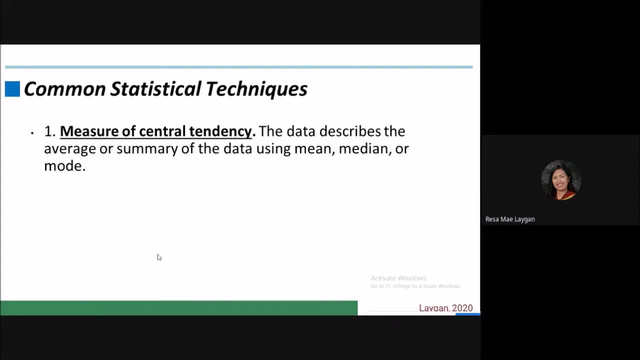 median. so in median, this is very good or very applicable, especially if you want to address the outliers or the data that is from far away from the center or from the common on data and or mode or the usual um data that you observe. no, from the observations. so that is for the measure. 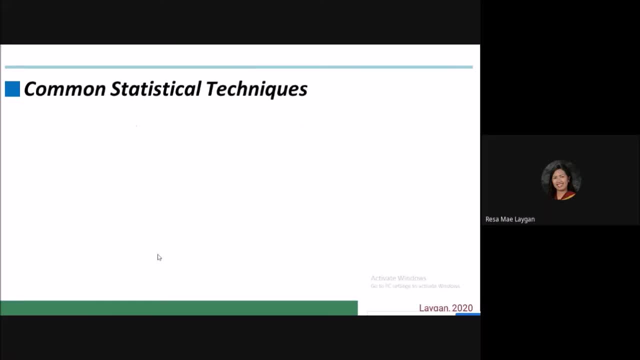 of central tendency, so another. in the higher statistical techniques we have parametric tests. so actually in parametric tests this test assumes that the data are on quantitative, numerical scale with a normal distribution of the underlying population. actually in the parametric test the data here are in continuous or 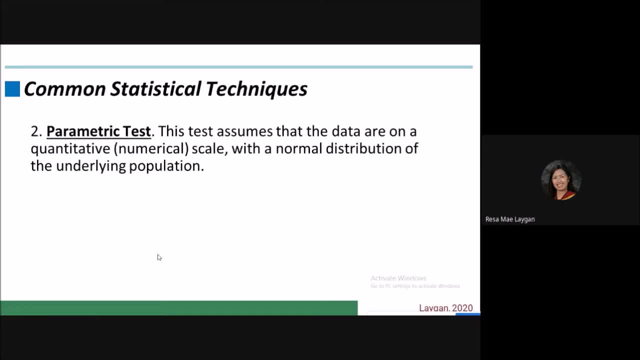 this involves continuous variables. so what are those continuous variables? for example, we have age now, because that is continuous variable, you can have from age one until age 100 or and so on, and also income. that is also a continuous variables or other quantitative or numerical scale. so under the parametric test we have the t-test. this is really common. 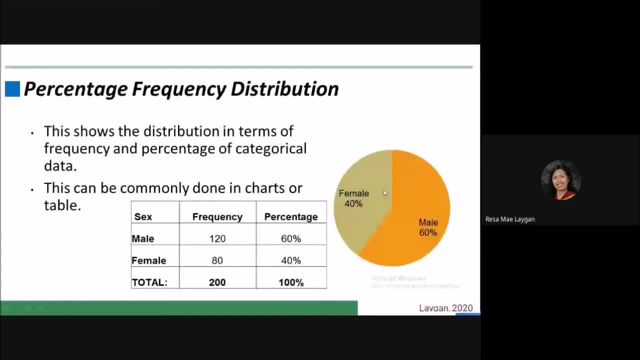 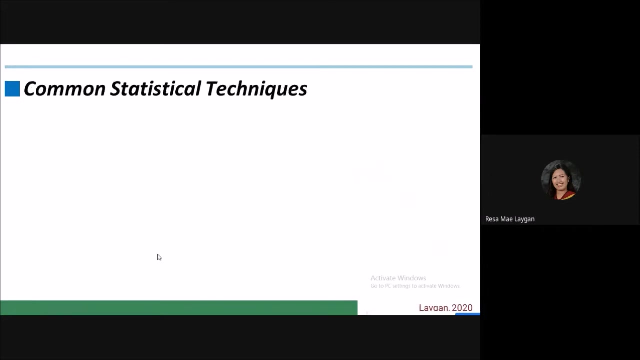 see the figure about the portion of each categorical data or you can use the table to summarize the frequency and the percentage distribution of each categorical data. so we have also common statistical techniques here and we have the measure of central tendency. so in the measure of central tendency the data describes the average of the data using mean median. 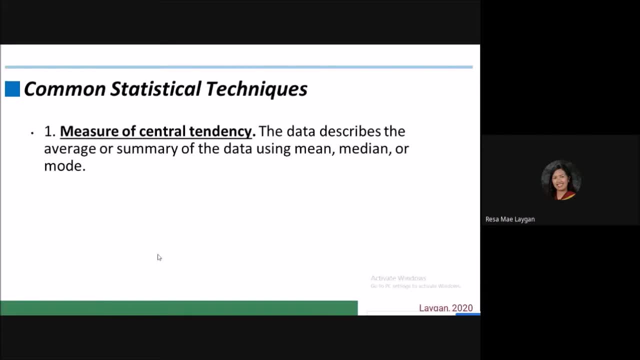 or mode, so these are familiar. so here you have to attest the center or the average. it can be a through the mean, no, or the average or the median. so in median this is very good or very applicable, especially if you want to address the outliers or the data that is from far away from the 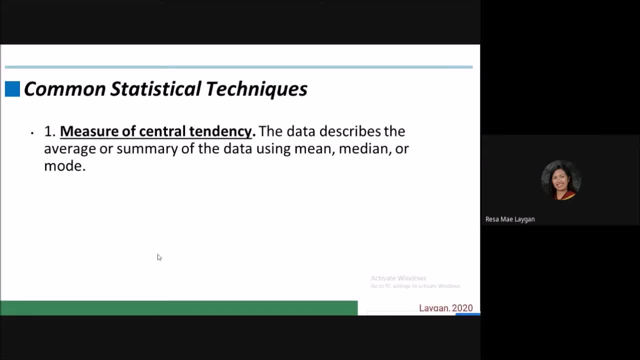 center, or from the common data and or mode or the usual data that you observe. no, from the observations. so that is for the measure of central tendency. so another. in the higher statistical techniques we have parametric tests. so actually in parametric tests, this test assumes that the data are on quantitative, numerical scale, with a normal 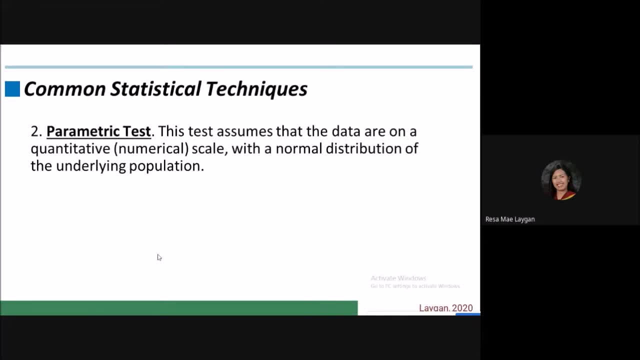 distribution of the underlying population. actually, in the parametric test, the data here are in continuous or this involves continuous variables. so what are those continuous variables? for example, we have age now, because that is continuous variable. you can have from age one until age 100 or and so on, and also income, that is also a continuous variables. or other. 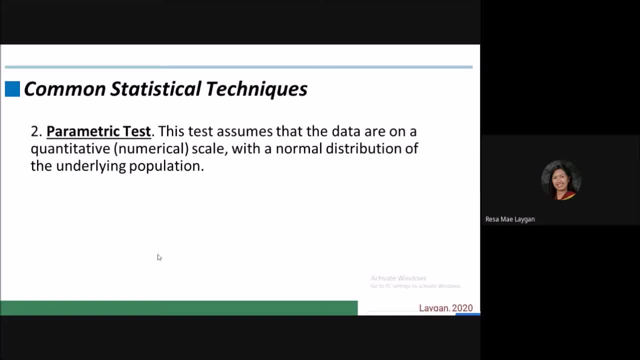 quantitative or numerical scale. so under the parametric test we have the t-test. this is really common and this t-test is used to test the null hypothesis, in which to determine if there is a no difference, especially the null hypothesis. now there is no difference between the means of the two groups. unfortunately, the disadvantage 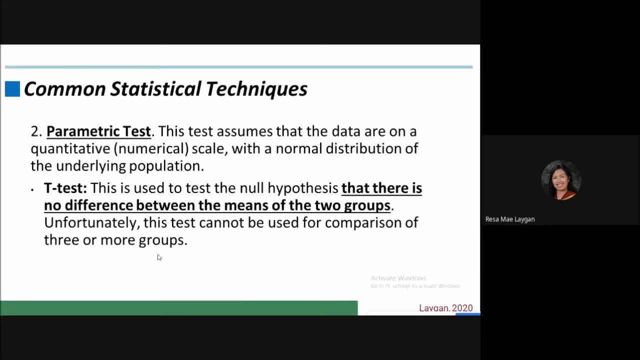 of t-test is that it cannot be used for comparison of three or more groups. so the focus here: it's very applicable only for the two groups, but in order to address or in order to compare three or more groups using this parametric test, we can use the analysis of variance or. 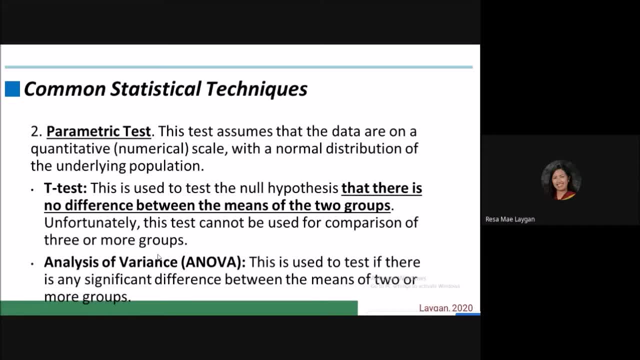 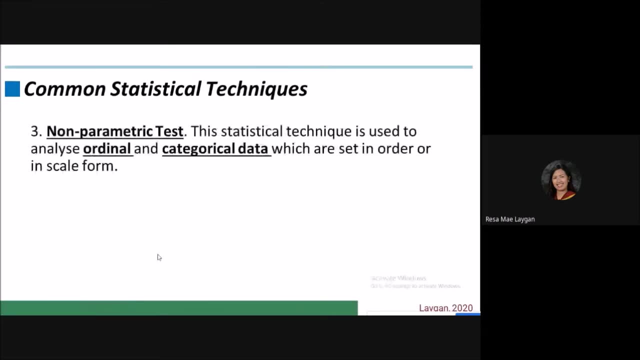 anova. so in anova this is used to test if there is any significant difference between the means of two or more groups. so that is for the analysis of variance or the anova. another, we have the non-parametric tests. so why is it non-parametric test? because the data that 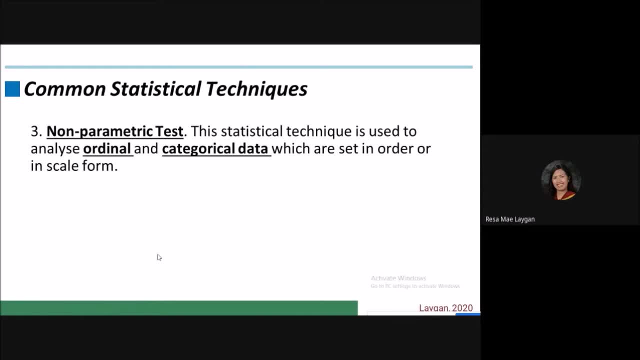 is being analyzed on this technique or on this test are not continuous data. unlike with the parametric test, they used to analyze continuous data here it used to analyze ordinal and categorical data, which are set in order for ordinal and category or in scale form for categorical data. 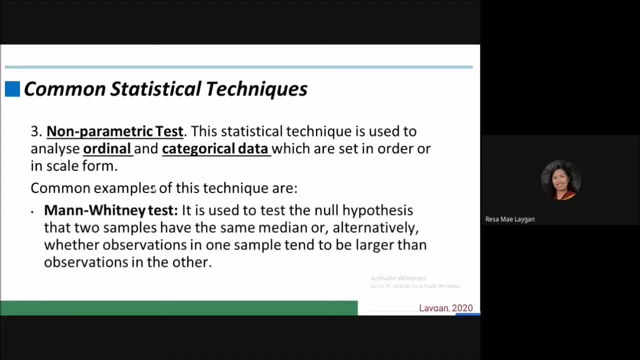 so the common example of this technique are the man whitney test versus the man whitney test. so in the man whitney test it is used to test the null hypothesis, by which the two samples have the same median, or alternatively, whether observations in one sample tend to be larger than observations in other. so that is for. 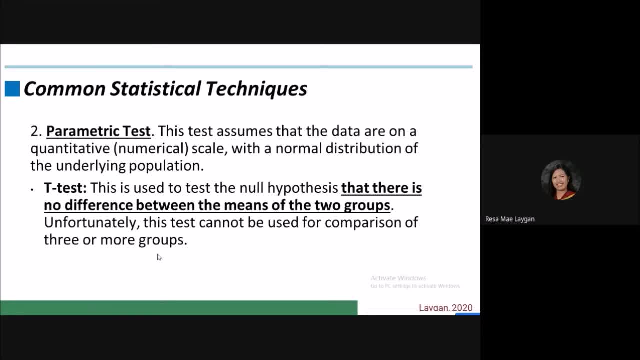 and this t-test is used to test the null hypothesis, in which to determine if there is a no difference, especially the null hypothesis. now, there is no difference between the means of the two groups. unfortunately, the disadvantage of t-test is that it cannot be used for comparison. 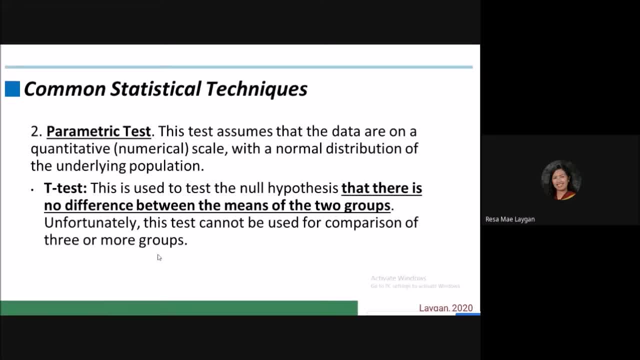 of three or more groups. so the focus here it's very applicable only for the two groups. but in order to address or in order to compare three or more groups using this parametric test, we can use the analysis of variance or ANOVA. so in ANOVA this is used to test if there is any. 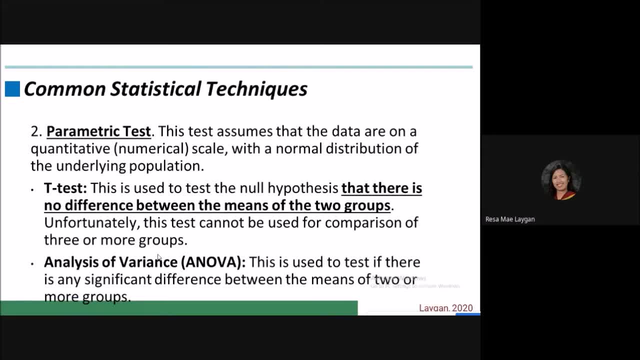 significant difference between the means of two or more groups. so that is for the analysis of variance or the ANOVA. another: we have the non-parametric test. this is used to test if there is any significant difference between the means of two or more groups. so that is for the analysis of variance or the ANOVA. 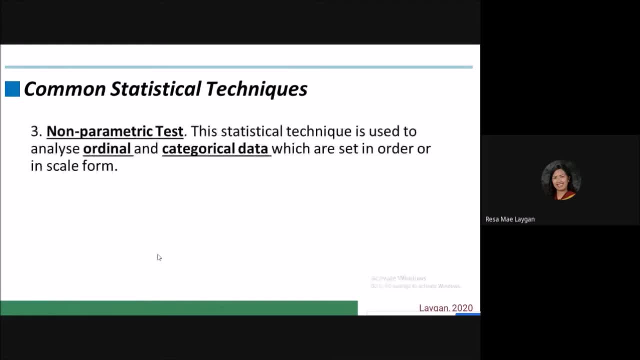 Another, we have the non-parametric tests. so why is it non-parametric? because the data that is being analyzed on this technique or on this test are not continuous data, unlike with the parametric test. they used to analyze continuous data. here. it used to analyze. 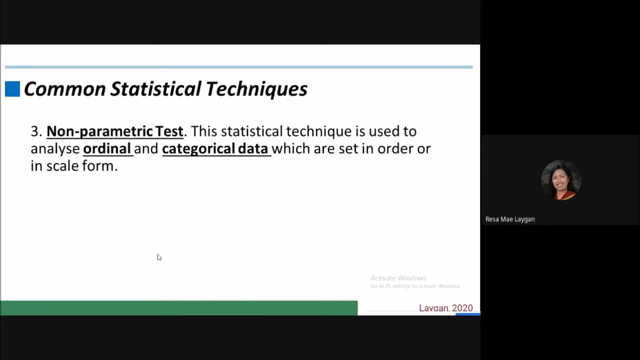 orginal and categorical data only for the non-parametric tests. In this example, the non-parametric test has 2 parameters: categorical data, which are set in order for ordinal, and category or in scale form for categorical data. So the common example of this technique are the Mann-Whitney test versus the 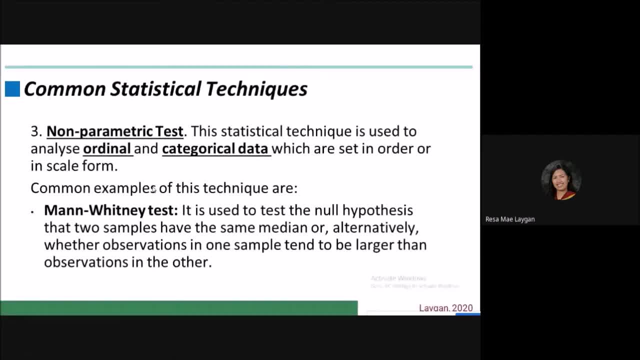 Mann-Whitney test. So in the Mann-Whitney test it is used to test the null hypothesis by which the two samples have the same median, or alternatively, whether observations in one sample tend to be larger than observations in other. So that is for the Mann-Whitney test. So actually this is more on. 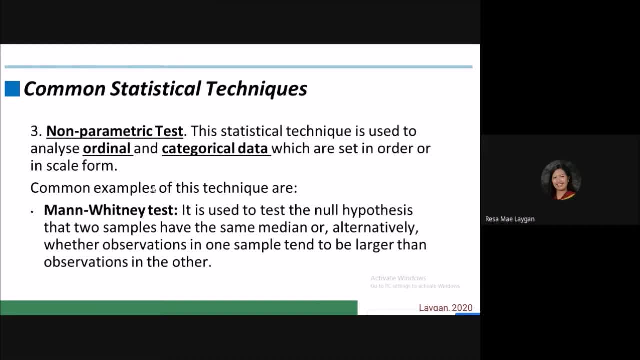 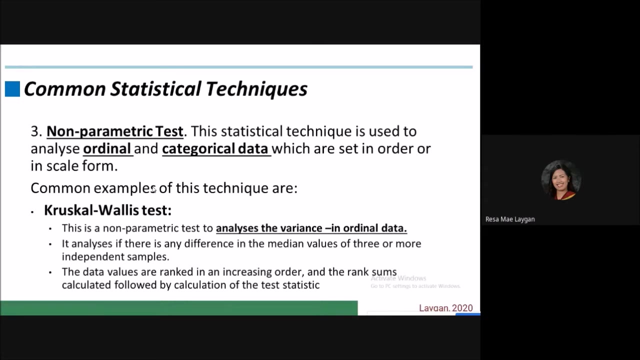 the man witness test with me test. so actually this is more on the two samples, or this is actually the version of the t-test, but on this it focuses on the ordinal or the categorical data. Kruskal Wallis test. so in Kruskal-Wallis test this is a non-parametric test. 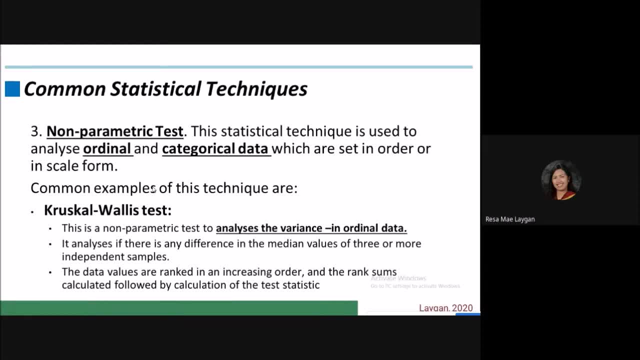 to analyzes the variants, but this is not in a continuous data but it is in ordinal data. so the data here are by in order. so it analyzes if there is any difference in the median data to satisfy the data. this is an experimental test and there will only be some. 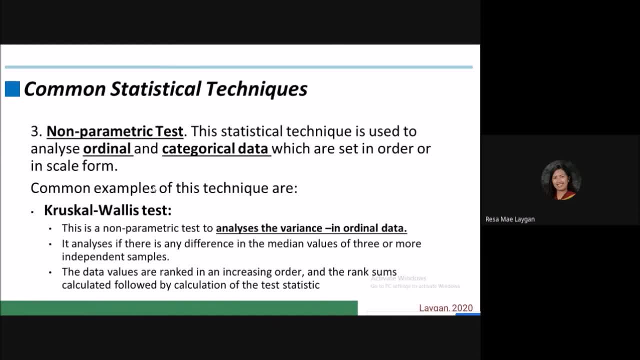 values of three or more independent samples, so the data values are ranked in an increasing order. because it involves ordinal data and the rank sums calculated, followed by calculation of the test statistic. actually, you can have this or you can get the result of this Kruskal-Wallis test. 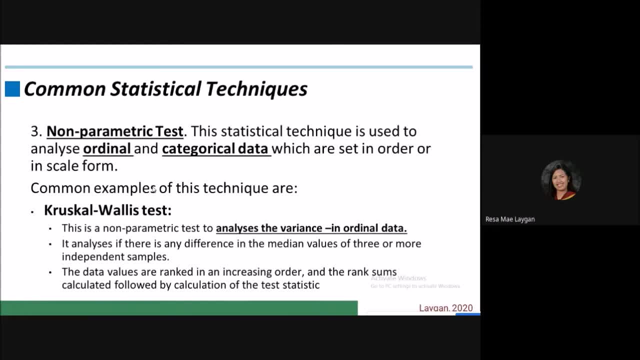 using the statistical tool, not just only on this test, but all of the statistical techniques can be obtained using a statistical tool and you have to make sure that you have a wide knowledge or the mastery in running those statistical tool and performing this series of statistical tests. or 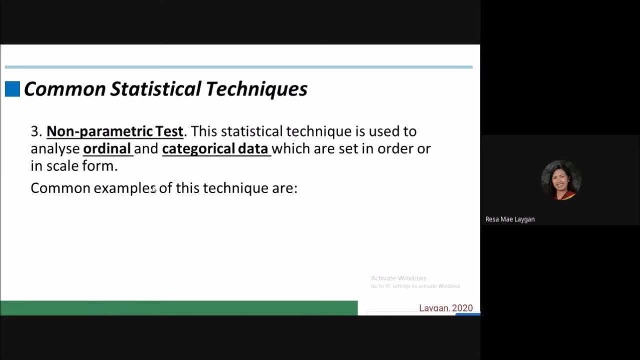 techniques and another and another. we have the Freidman test. so this is a non-parametric test for testing the difference between related samples. the Freidman test is actually an alternative for repeated measures, ANOVAs, which is used when the same parameter has been measured under different conditions. on the 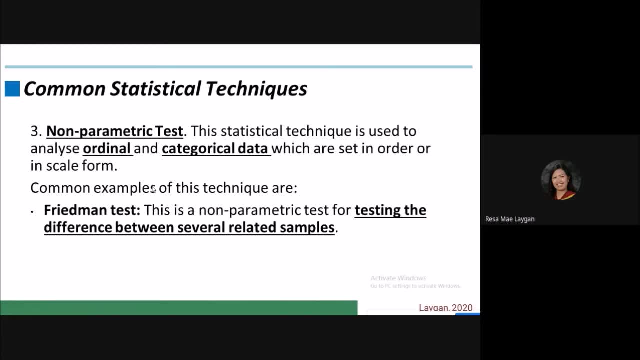 same test unit subjects. so that is for the Freidman test and other non-parametric technique is we have the Spearman rank test. actually, the Spearman rank test is the same with the correlation analysis by which you test the strength of a link between the two sets of the categorical data variables. this is actually. 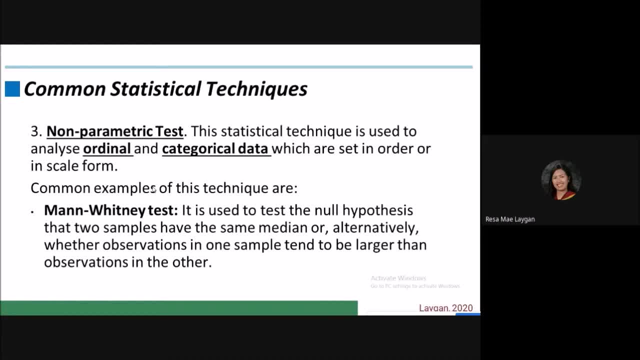 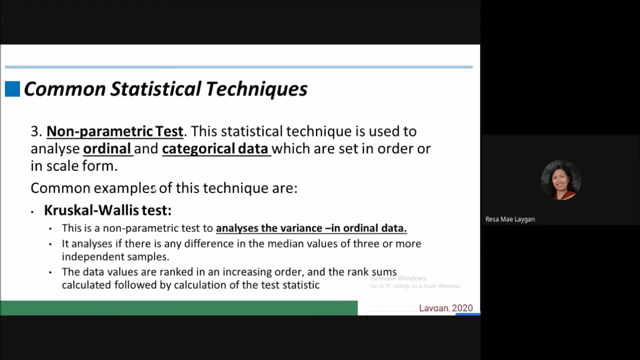 the two samples, or this is actually the version of the t-test, but on this it focuses on the ordinal or the category Croscal-Wallis test. So in Croscal-Wallis test this is a nonparametric test to analyze the variance. So, but this is not in a continuous data, but it is in ordinal data. So the data here are by: 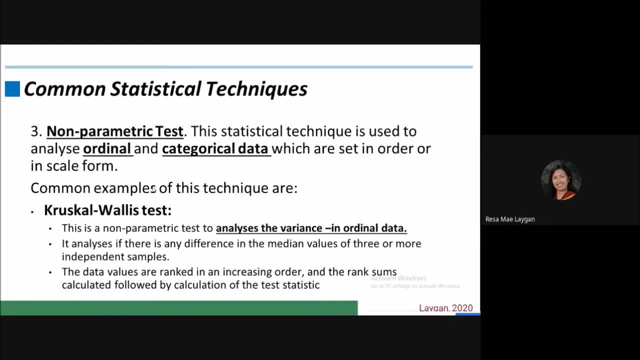 in order. So it analyzes if there is any difference in the median values of three or more independent samples. So the data values are ranked in an increasing order because it involves ordinal data and the rank sums calculated, followed by calculation of the test statistic. Actually, you can have this or you can get the result of this. 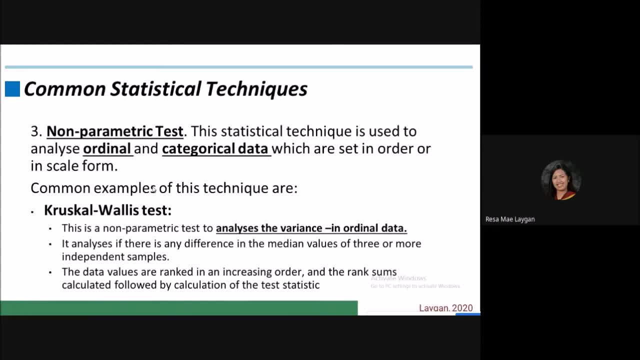 Croscal-Wallis test using the statistical tool, Not just only on this test, but all of the statistical techniques can be obtained using a statistical tool and you have to make sure that you have a wide knowledge or the mastery in running those statistical tool and performing this. 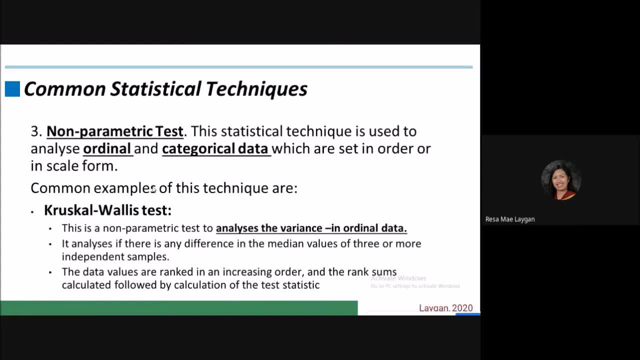 series of statistical tests or techniques, And another and another. we have the Freidman test. So this is a nonparametric test for testing the difference between related samples. The Freidman test is actually an alternative for repeated measures, ANOVAs, which is used when the 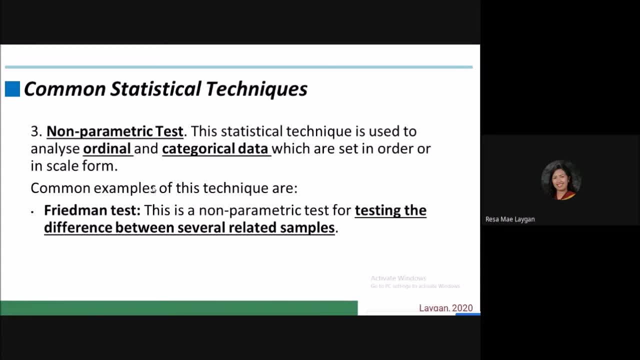 same parameter has been measured under different conditions on the same subjects. So that is for the Freidman test And other nonparametric technique. is we have the Spearman rank test? Actually, the Spearman rank test is the same with the correlation analysis. 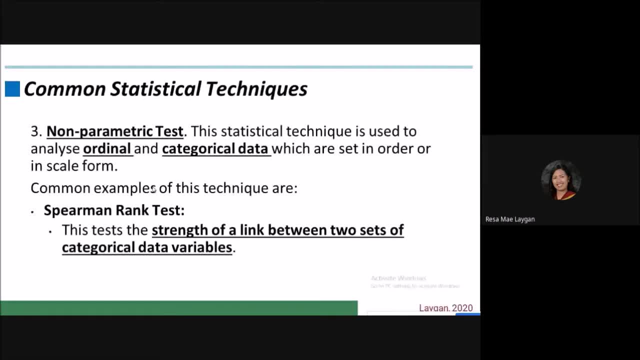 by which you test the strength of a link between the two sets of the categorical data variables. This is actually applicable if your data are more on Likert scale and you want to examine the link between the two variables by which their data sets are in Likert or by which these 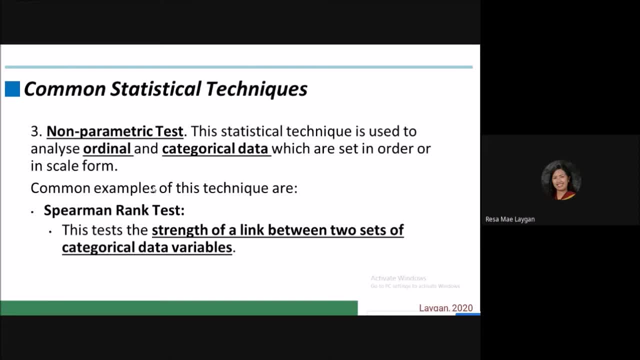 two variables are in categorical data or in Likert scale, For example, we have the level of awareness and the the practices. So, for example, so you obtain the data of these two variables variables, we have the level of awareness, which is your independent variable, and the practices, or 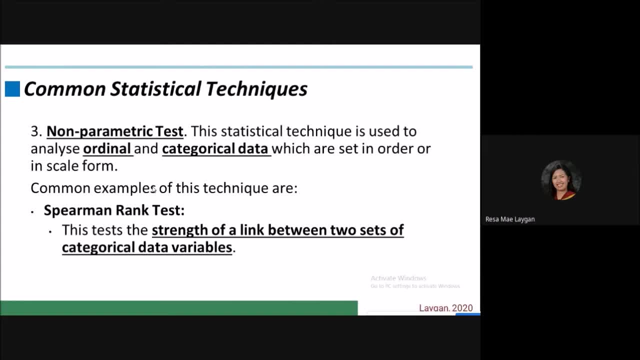 level of practices, which is your dependent variable and you want to to test the strength, the link between these two variables and these variables. you obtain this using a Likert scale, or thus the data for this variables are in categorical data, so you may apply Spearman rank test in testing the strength or the link or the relationship if there is a significant. 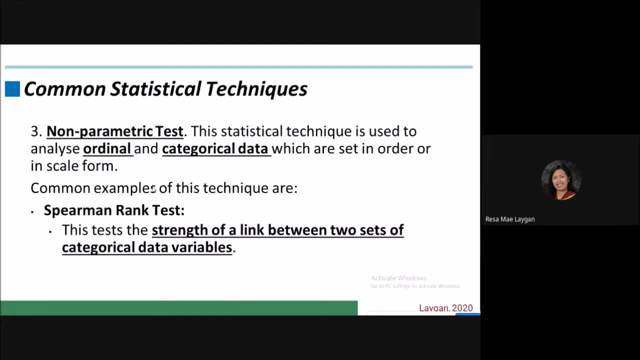 relationship, or the relationship is positive or negative between the level of awareness, which is a categorical data and your independent variable, and the practices, which is your dependent variable and has the categorical data. so that is where you apply the Spearman rank test. so another common statistical techniques here is we have the 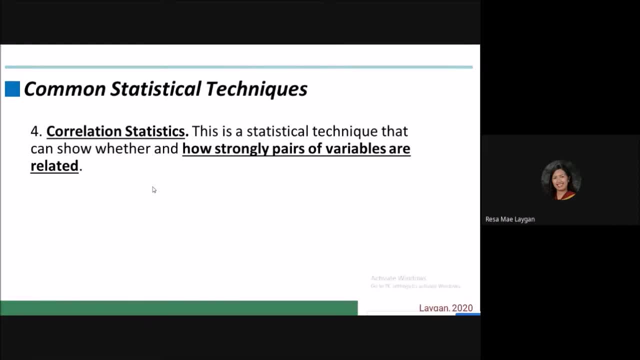 correlation statistics, and this is very common. so actually this is a statistical technique that can show whether and how strong the relationship between the level of awareness and the strength pairs of variables are related. the same with the Spearman Spearman rank test, but the difference is that in the Spearman rank test its focuses on the categorical data, here under the correlation. 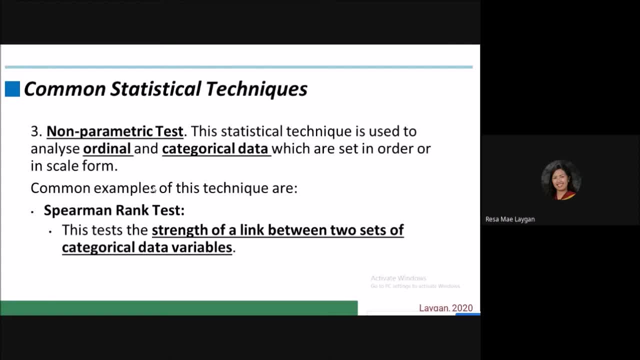 applicable if your data are more or less in the same category than the other data variables. more on Liker and you want it to examine the link between the two variables by which their data sets are in Likert or by which the variables are categorical data. for example, we have the level of awareness. 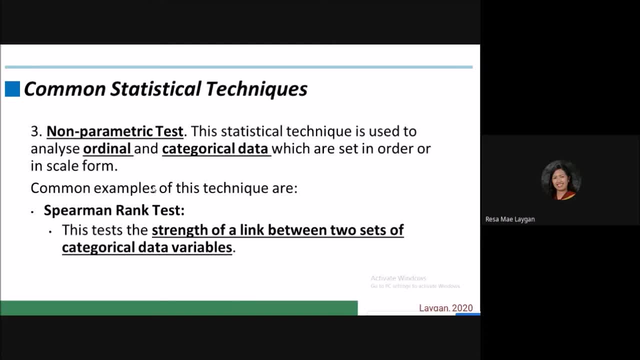 and the practices. so we all have the level of awareness. Ewriter, our normal protocol using the same enumeration: e- ansaw〜 for counter print taunt narration. So, for example, so you obtain the data of these two variables: we have the level of awareness, which is your independent variable, and the practices, or level of practices, which is your dependent variable. 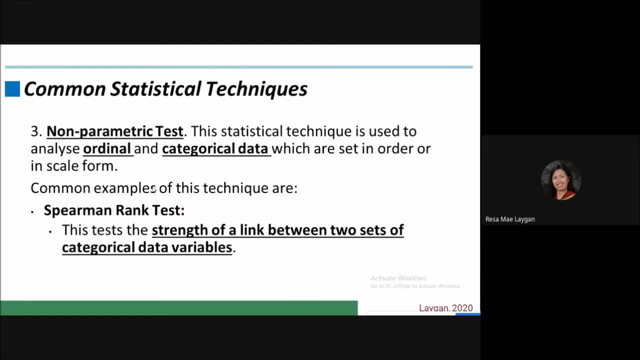 And you want to test the strength, the link between these two variables And these variables. you obtain this using a Likert scale, or thus the data for these variables are in categorical data. So you may apply Spearman-Rung test in testing the strength or the link or the relationship. 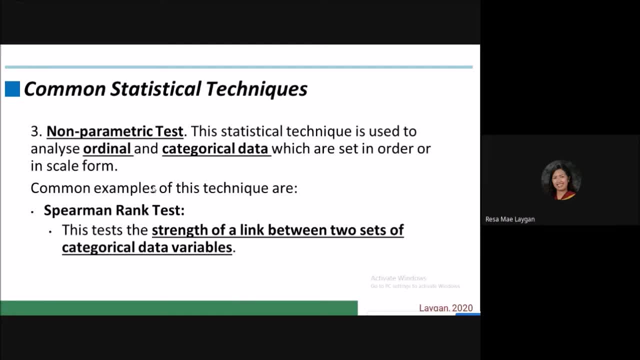 If there is a significant relationship or the relationship is positive or negative between the left- The level of awareness, which is a categorical data, and your independent variable- and the practices, which is your dependent variable and has the categorical data. 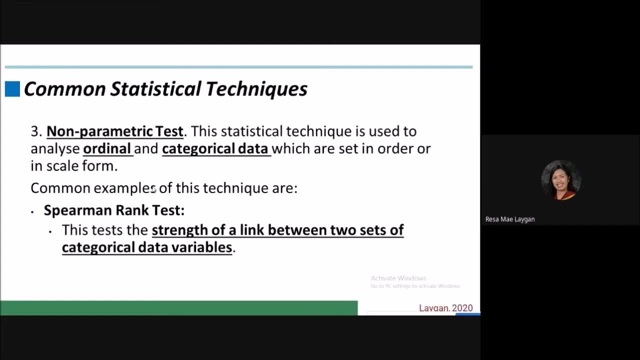 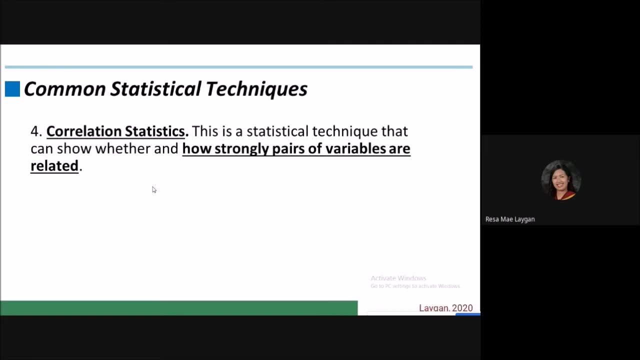 So that is where you apply the Spearman-Rung test. So another common statistical technique here is: we have the correlation statistics And this is very common. So I Actually this is a statistical technique that can show whether and how strongly pairs of variables are related. 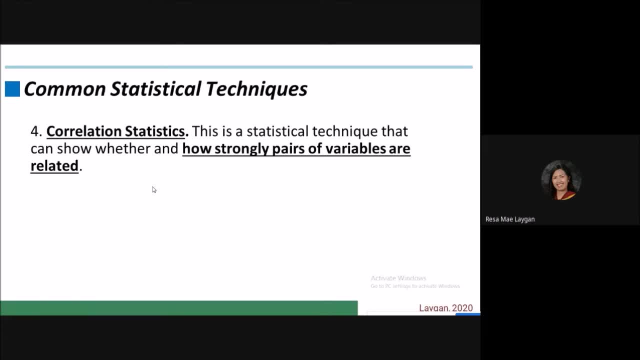 The same with the Spearman-Rung test, but the difference is that in the Spearman-Rung test it focuses on the categorical data. Here, under the correlation statistics, it shows how strong relationship of the variables no, Or how strongly pairs. 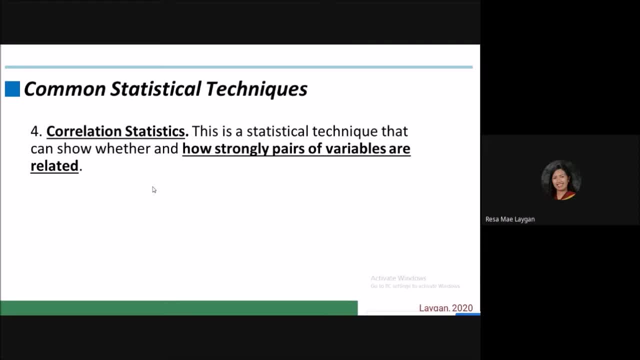 statistics it shows from how strong relationship of the variables know or how strongly pairs of variables are related. and under this is we have the person's correlation and the person's correlation. so in the person's correlation this test the statistical relationship or association between two continuous variables. take note, it's not categorical data variables but two continuous. 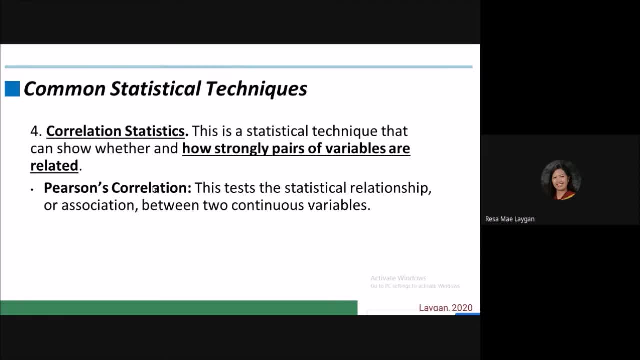 variables. so, for example, we have age, but sometimes also age can be categorical data. that it depends on how you get the data. so if there is no limit or there is no category in determining age, then you can use no age as your continuous variables, for example, 16, 17, 18 and so on. if you 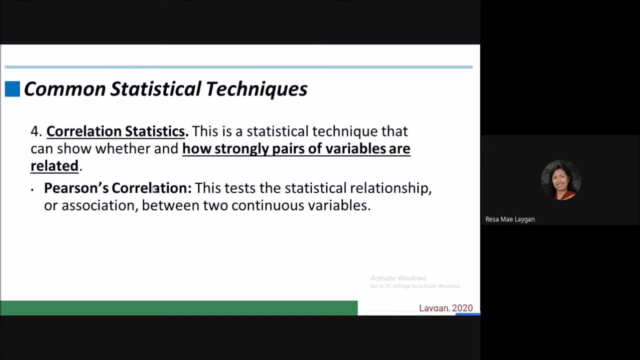 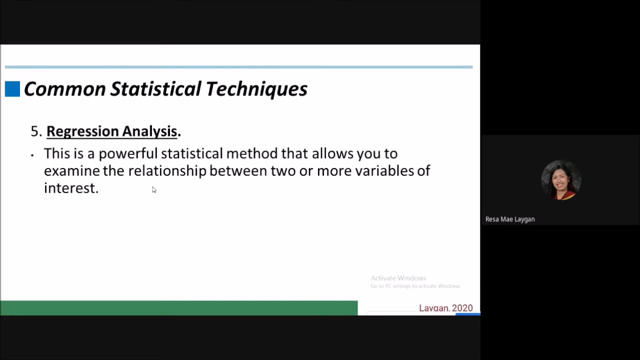 obtain the age using the categorical data, like, for example, old, young- that is categorical data. then you may use the Spearman rank test, so here it is applicable for the continuous variable- and lastly, test the regression analysis. actually, the regression analysis is a powerful statistical method that 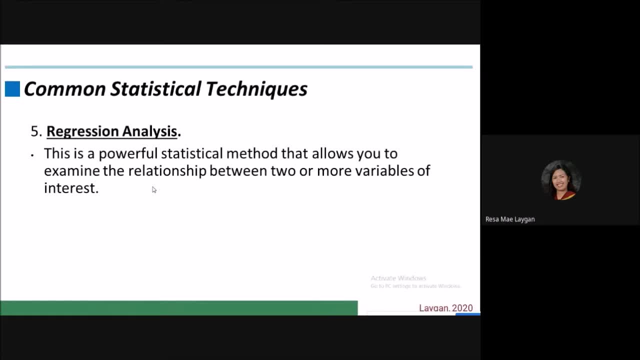 allows you to examine the relationship between two or more variables of interest. so this examines the influence or effect of one or more variables on a independent or a dependent variable. so this examines the influence or effect of one or more jargon 너 more independent variables on a dependent variable. So if your study wants to assess the effect, 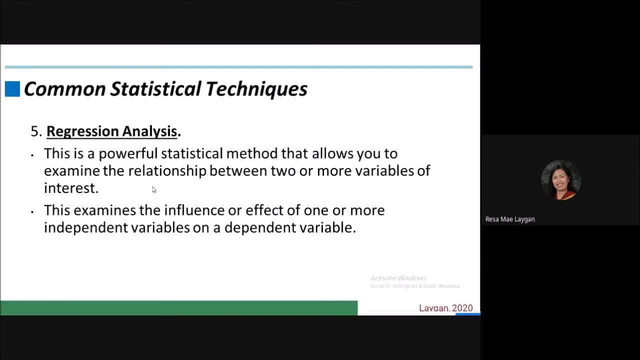 of this independent variable on dependent variable, or if you want to examine the influence of this variable to another variable, or if you want to assess the factors influencing this dependent variable, then regression analysis is the best tool that, or the best technique that you may use. So 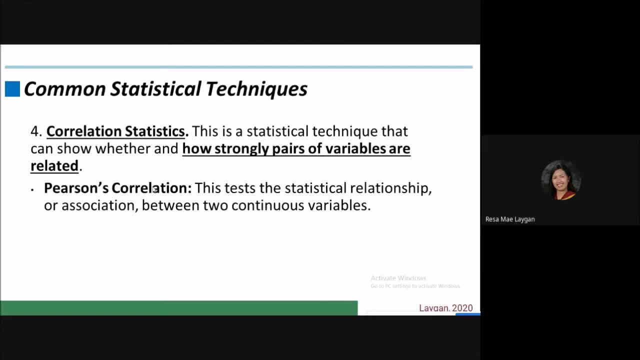 Of variables are related And under this is we have the person's correlation. So in the person's correlation this tests the statistical relationship or association between two continuous variables. Take note, it's not categorical data variables but two continuous variables. 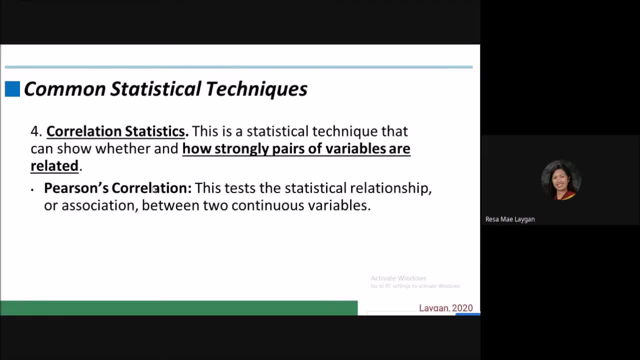 So, for example, we have age, but sometimes also age can be categorical data. it depends on how you get the data. So if there is no limit or there is no category in determining the age, then you can use age as your continuous variables. 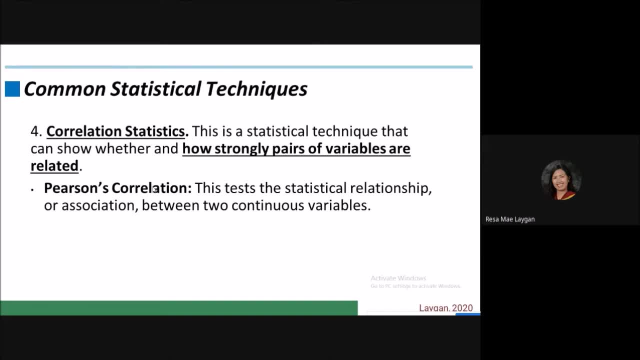 For example, 16,, 17,, 18, and so on. If you obtain the age using the categorical data, like for example, old, young- that is categorical data- then you may use the Spearman-Rung test. So here, 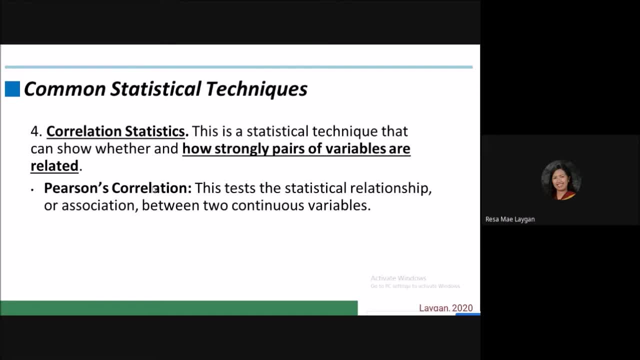 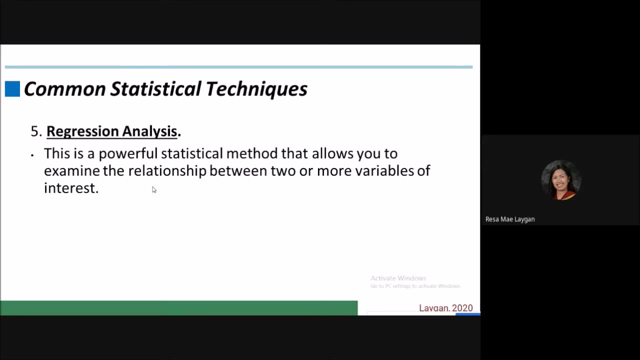 It is applicable for the continuous variable. And lastly, we have the regression analysis. Actually, the regression analysis is a powerful statistical method that allows you to examine the relationship between two or more variables of interest. So this examines the influence or effect of one or more variables on a independent. 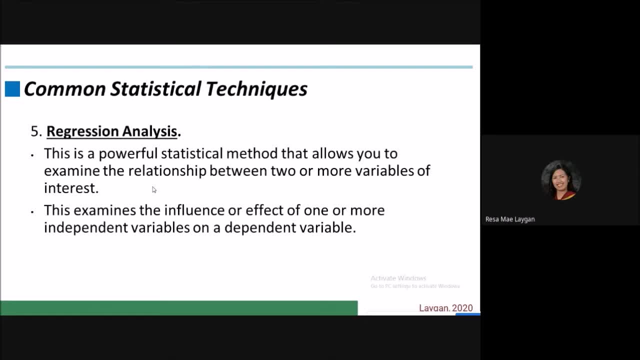 Or a dependent variable. So this examines the influence or effect of one or more independent variables on a dependent variable. So if your study wants to assess the effect of this independent variable on a dependent variable, or if you want to examine the influence of this variable to another variable, or if you want to assess the factors supporting a dependent variable on another variable, or what was the same one ineffective, lame. 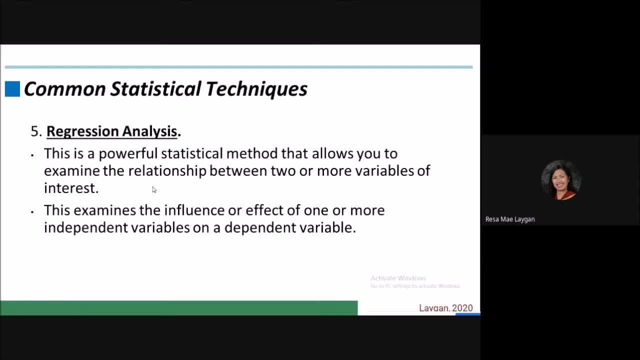 quantities and so on. This Untersize 3D__ 食べ é, and that is it, Thank you. Thank you, you're welcome. Bye, Okay, Goodbye. influencing this dependent variable, then regression analysis is the best tool. that, or the. 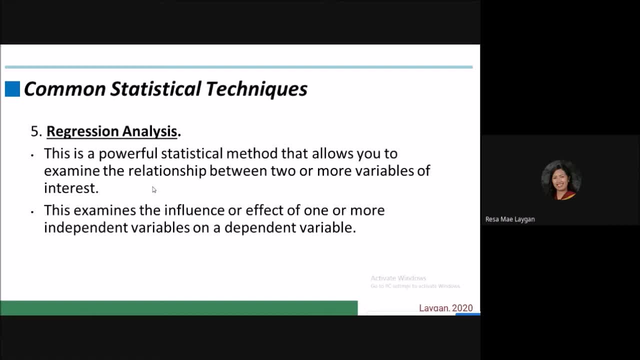 best technique that you may use. so, actually, there are various, not types of regression analysis, depending on the data and on the state of the problem that you want to assess. so, actually, if you are going to use the ols or the ordinary, ordinary, least square regression, then you have 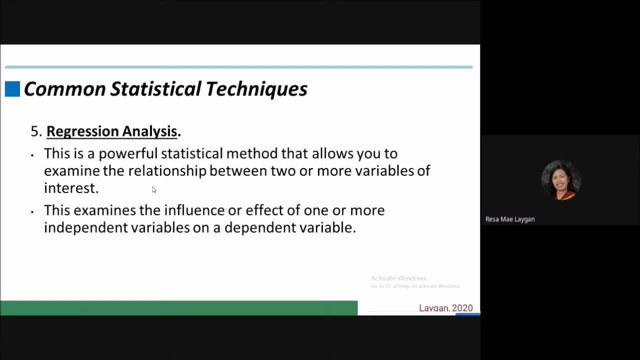 to obtain data more than 30, and also it depends on how many parameters that you are going to use, because the degree of freedom is also um related on that. but there are also regression analysis or types of other types of regression that can use to address data which are less than 30 and especially this data are in time series, so you can use the arima. 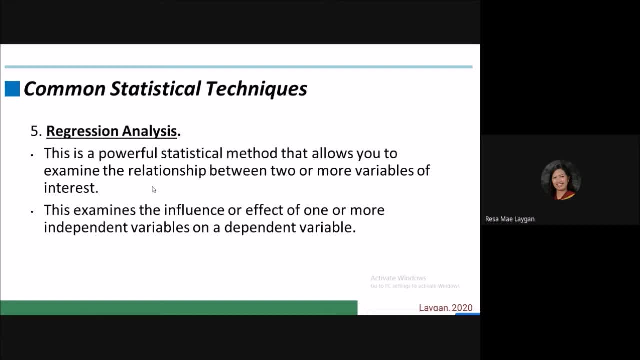 for the univariate analysis, or you may use the bar or the vector autoregressive for the multivariate, and i here on this video, i'm just only focusing on the overview, only on what statistical techniques you are going you may employ in your research. so these are basic only. so there are other types. we 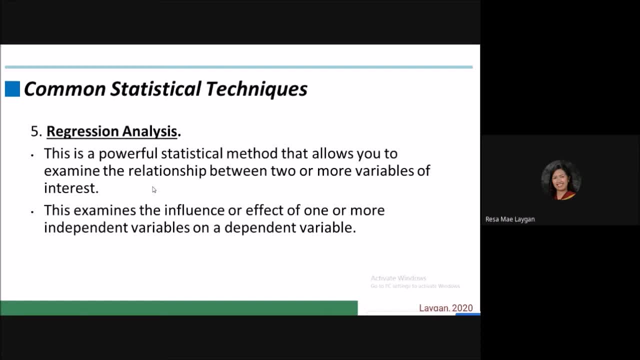 have also factorial analysis. we have also structural equation modeling. we can apply also those- and this video is limited long- only in the regression analysis and those other statistical techniques that have mentioned. but in order to more, to know this more, i will show you the five key assumptions under this analysis. so in use if you wish to use this. 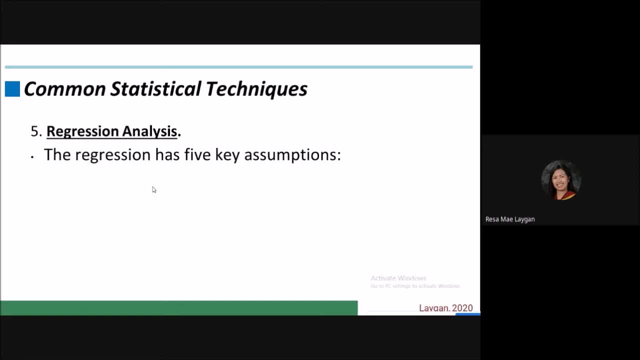 analysis or this type of statistical technique. you have to ensure that your model underlies, on this, five key assumptions. so you have to make sure that the relationship of your independent and dependent variable is linear, so the linearity assumption can be tested with scatter plots. and another assumption is that we have this multivariate normality. 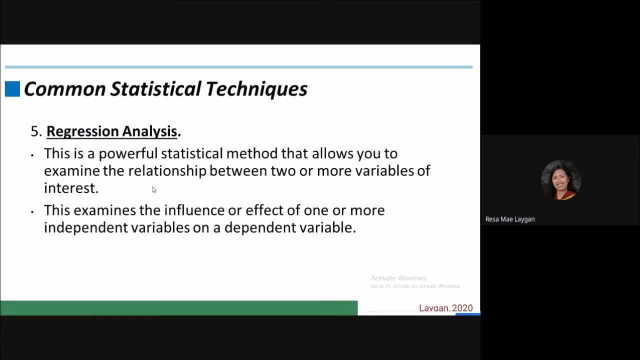 actually there are various, not types of regression analysis, depending on the data and on the statement of the problem that you want to assess. So, actually, if you are going to use the OLS or the ordinal, ordinal list square regression, then you have to obtain data more than 30, and also it depends on how many. 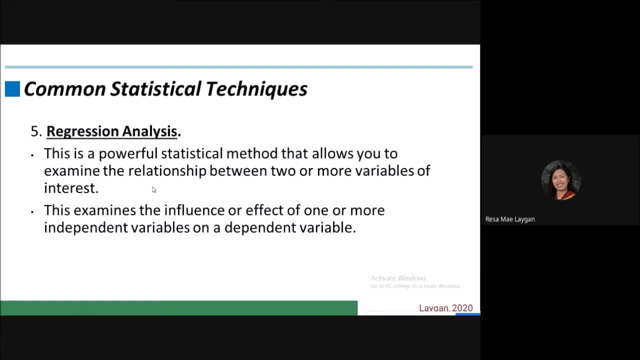 parameters that you are going to use, because the degree of freedom is also related on that. But there are also regression analysis or other types of regression that can use to address data which are less than 30. Especially, this data are in time series, So you can use the arima or the univariate analysis or you may use the. 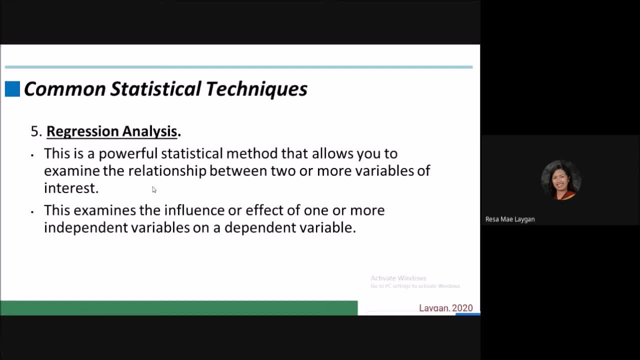 bar or the vector autoregressive for the multivariate. And I am here on this video, I'm just only focusing on the overview, only on what statistical techniques you are going you may employ in your research. So we will continue with the analysis and we will see you in the next video, Thank you. 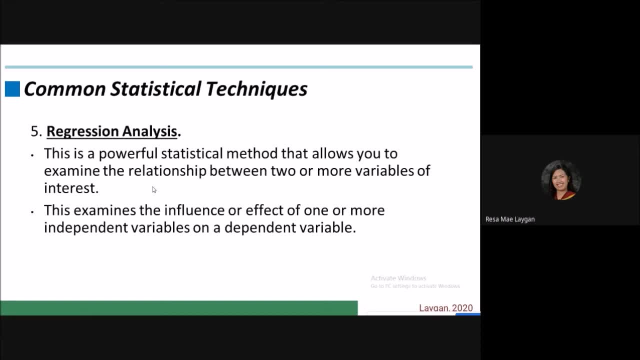 So these are basic only. So there are other types. We have also factorial analysis. We have also structural equation modeling. We can apply also those- And this video is limited only in the regression analysis and those other statistical techniques that have mentioned. But in order to know this more, I will show you the five key assumptions under this analysis. So if you wish to use this analysis or this type of statistical technique, you have to ensure that your model underlies on these five key assumptions. 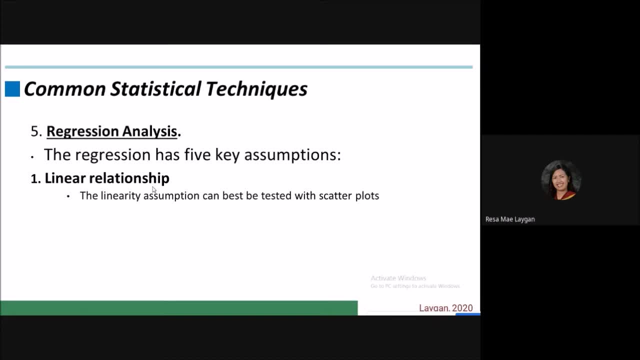 So you have to make sure that the relationship Of your independent and dependent variable is linear. So the linearity assumption can be tested with scatter plots. And another assumption is that we have this multivariate normality. This means that your data should be in normal distribution And you have to address also the outliers. 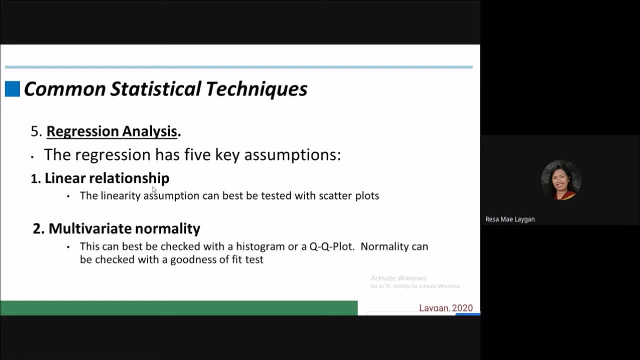 this means that your data should be in normal distribution and you have to address also the outliers and also you can- this can be best- the check with a histogram or the qq plot so to attest the if, the, if the um, this variable or certain variable is positively skewed or negatively skewed. 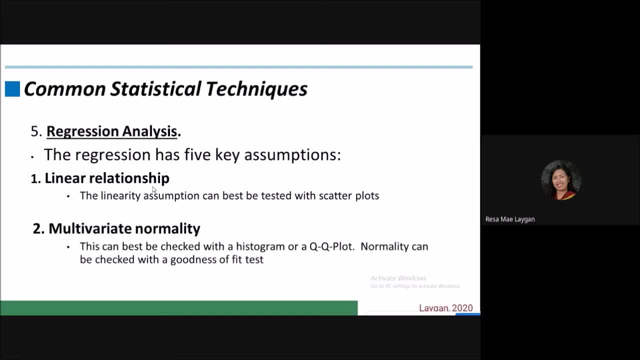 then we will decide if we need to transform this variable into log form or into exponential form. and actually the normal can be checked with a goodness of fitness, and there are various of goodness of fitness that can check the normality of your data. another is we have the no or little multi-coloniality. 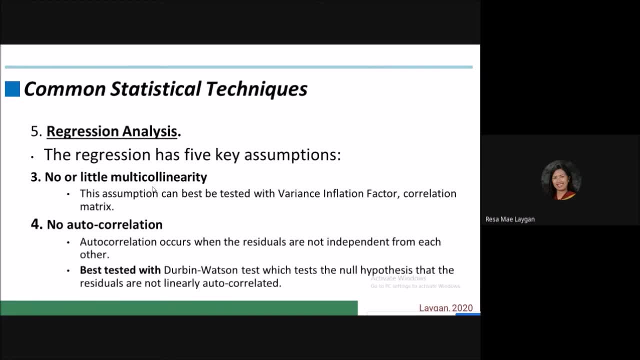 so actually, multi-coloniality exists, and this is a phenomenon by which one predictor variable in a regression model can be linearly predicted from the others with a substantial degree of accuracy. so if your um model or the multi-coloniality issue of that model, 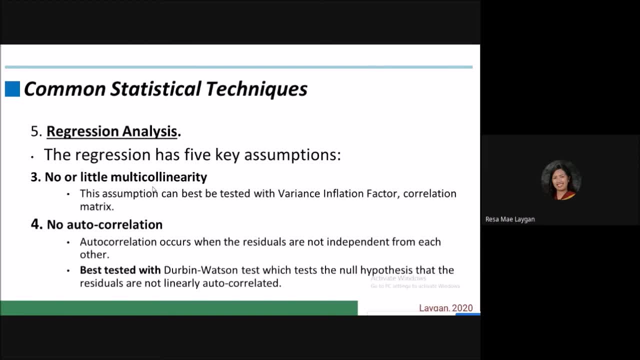 is very serious. then there is a one um, there is a possible implication on the in estimating the coefficient now of that regression model and may change erratically in response to small changes in the model or the data. and actually the multi-coloniality does not. 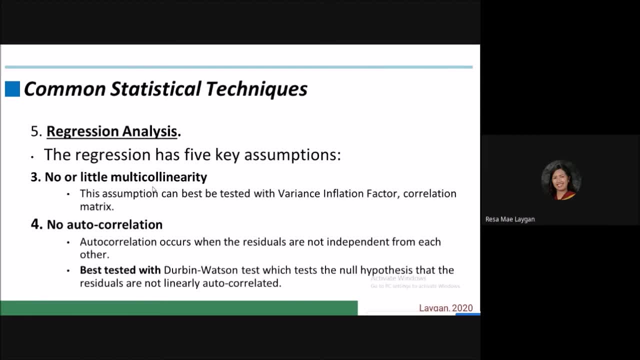 reduce the predictive power or the relay reliability of the model as a whole, but at least within the sample data set. it only affects the calculation with regards to the individual predictors and actually this assumption типа variance inflation factor and correlation matrix um, it shows these. for example, this very important variable is highly correlated. 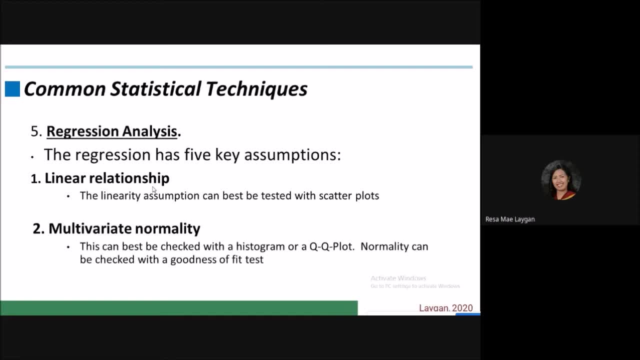 And also You can. This can be best checked with a histogram or the QQ plot. So to attest the, if the, if the this variable or certain variable is positively skewed or negatively skewed, then we will decide if we need to transform this variable into log form or into exponential form. 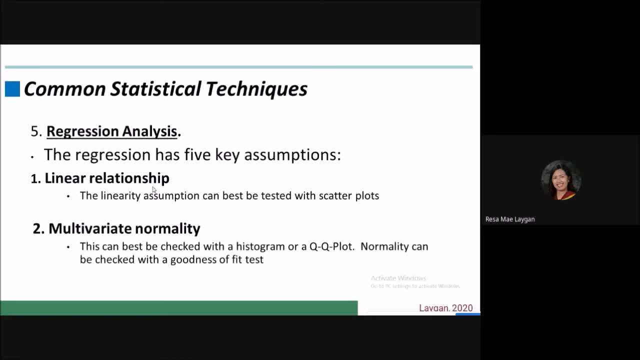 And actually the normality can be checked with a good normality. So this is a thing that, because you existed, you can check the essentially the normality of the data and it gets going along with a simple graphs, And then theimer is the well known numerator. 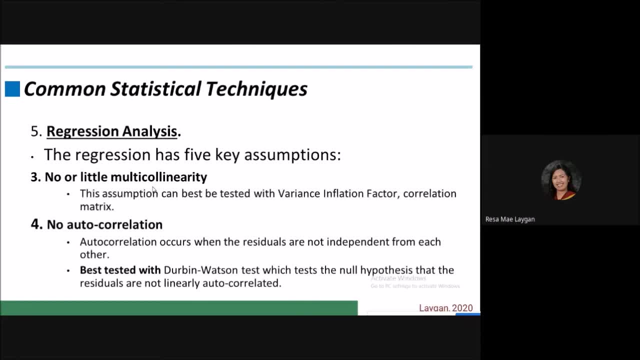 And what you'll see in this. Similarly, there are various of fitness. There are various of goodness of fitness that can check the normality of your data. Another is we have the no or little multicultural æ. So actually multicultural æ exists and 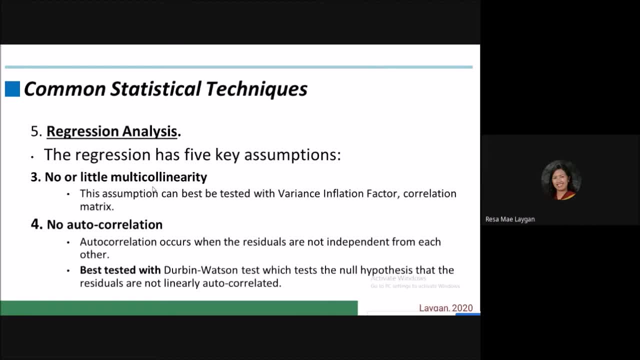 This is a phenomenon by which one predictor variable in regularize is expressed in a nonlinear class, And this is the case If we have a nonlinear data method for the nonlinear graph With, let's say, I will call it linear Olaf's Seas. 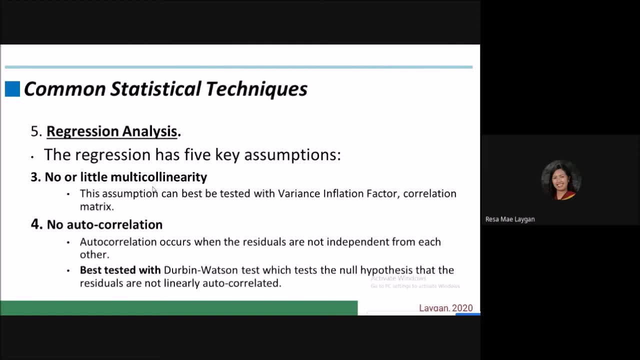 When you haveliamo P7. model can be linearly predicted from the others with a substantial degree of accuracy. so if your model or the multi-core collinearity issue of that model is very serious, then there is a one. there is a possible implication on the estimating the coefficient now of that regression model and 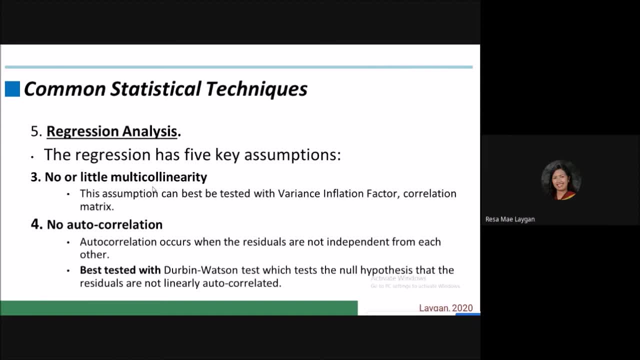 may change radically in response to small changes in the model or the data. and actually the multi collinearity does not reduce the predictive power or the relay reliability of the model as a whole, but at least within the sample data set it only affects the model as a whole. so the model is 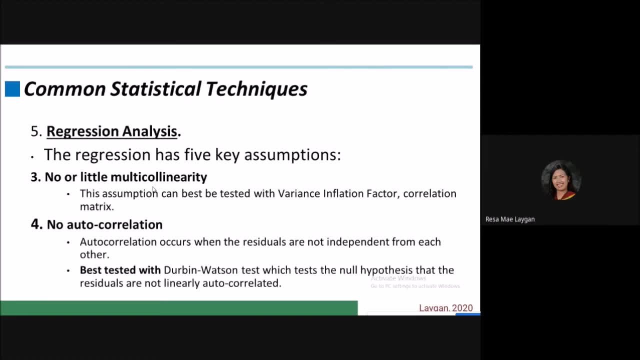 a calculation with regards to be individual predictors and actually this assumption can be best tested with variance inflation factor and correlation matrix. in multi collinearity casse. it shows these, for example. this variable is highly correlated with this other independent variable so for the same reason, it may be best tested with variance inflation factor and correlation. 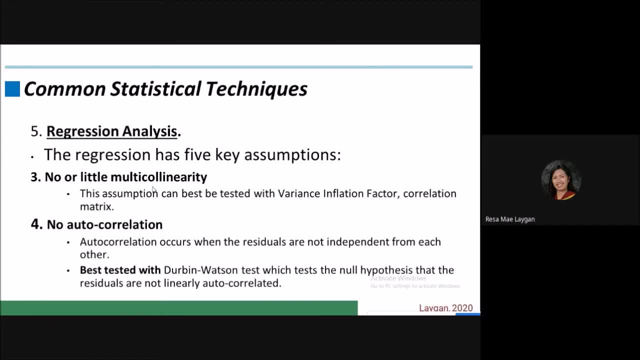 with this other independent variable. so, for example, you have the population m- a survival population. if you would consider the population as your variable, this corpses in efter, etc. you another is- is highly correlated with the being of this other independent variable. so, for example, you the population, a survival variable is very закончing the relates. 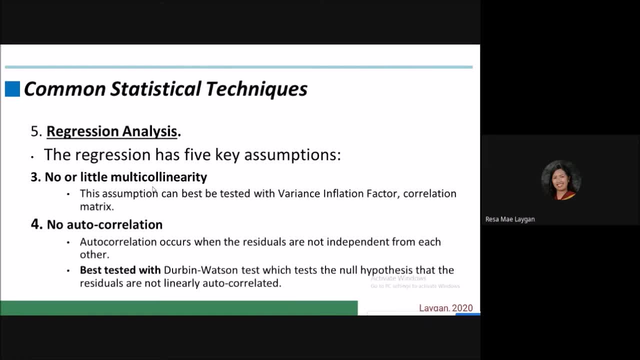 and you have also the another variable, independent variable, which is population growth. I think the population and population growth is somehow are highly related. On this, you have to omit either the population variable or the population growth in order to address the multi-collinearity issue. We have the no autocorrelation. so in when we say: 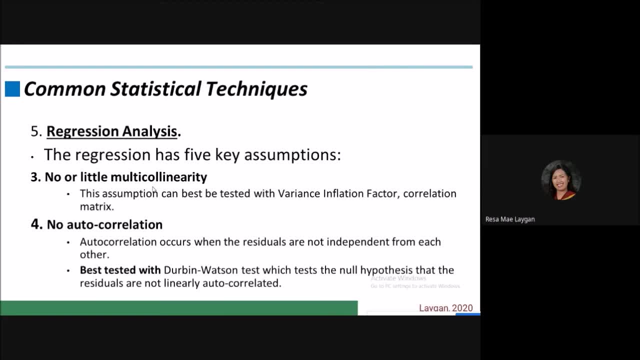 autocorrelation. it occurs when the residuals are not independent from each other. In testing the autocorrelation it can be best tested with Durbin-Watson test, which it tests the null hypothesis that the residuals are not linearly autocorrelated. So when we say autocorrelated, so the correlation. 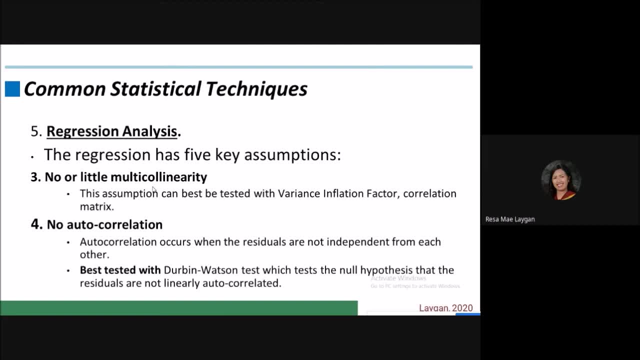 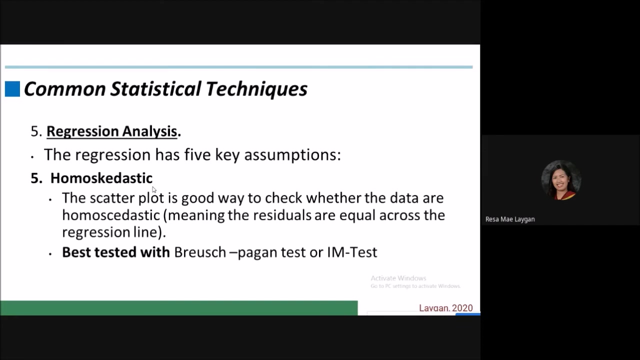 between the elements of a single of data, or these variables are almost the same and others from the series separated from them by a given interval. and lastly, we have the assumption of homoscedastic. so when we say homoscedastic it is equal variance in measuring the homoscedastic. actually, scatter plot is good. 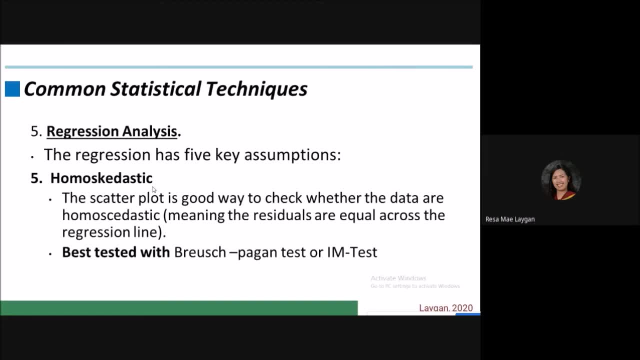 way to check whether the data are homoscedastic or equal across the regression line. and actually it is somehow related with the normality of the distribution of your data variables in a certain plot. so this can be best tested with brush pagan test. this is actually a diagnostic test for 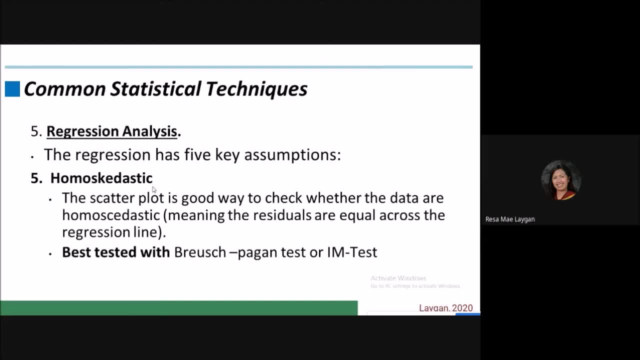 testing, the homoscedasticity and the IM test. so actually in homoscedasticity it describes a situation in which the error term or the disturbance of your model or the random disturbance in the relationship between the independent variables and dependent variable is the same across all values of the independent. 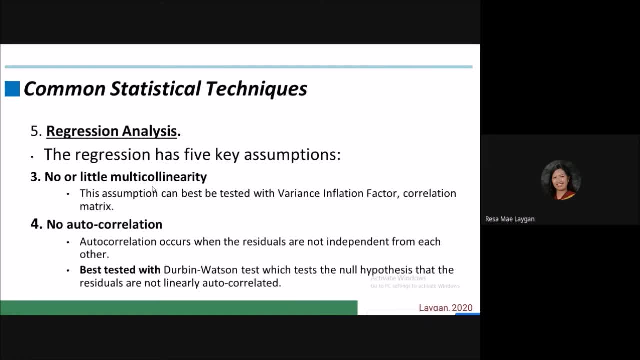 For example, you have the population as your variable and you have also the another variable, independent variable, which is population growth. I think the population and population growth is somehow are highly correlated. On this, you have to omit either the population variable or the population growth in order to address the multicollinearity issue. 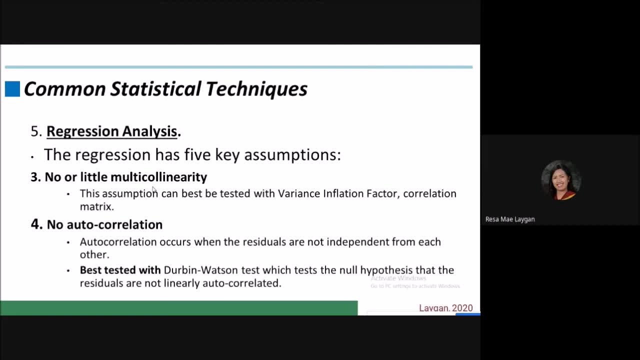 We have the no autocorrelation. So when we say autocorrelation it occurs when the residuals are not independent from each other. In testing the autocorrelation it can be best tested with Durbin-Watson test, which it tests the null hypothesis that the residuals are not linearly autocorrelated. 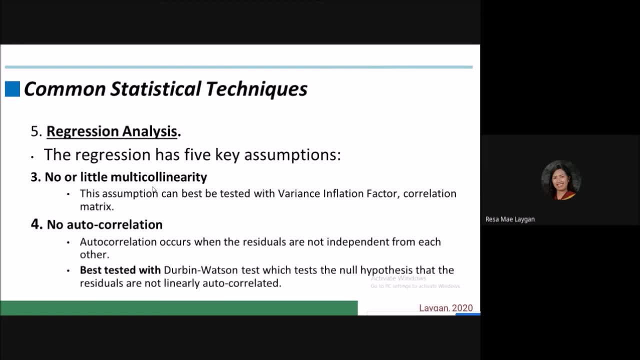 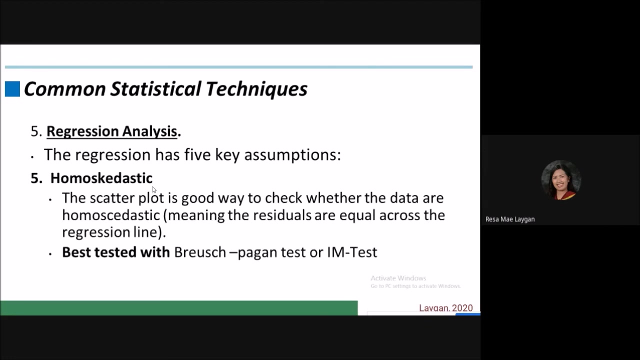 So when we say autocorrelation, so the correlation between the elements of a series of data or these variables are almost the same and others from the series separated from them by a given interval. And lastly, we have the assumption of homoscedastic. 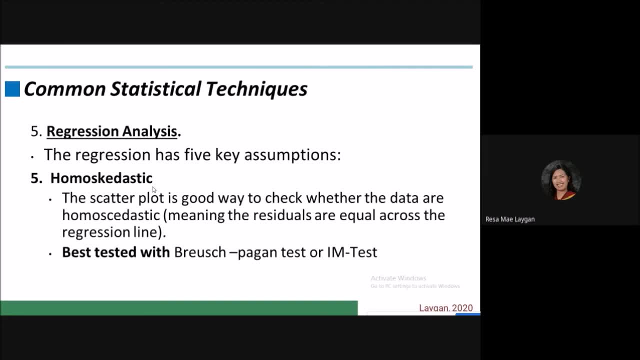 So when we say homoscedastic, it is equal. So this is the most common variance In measuring the homoscedastic. actually, scatterplot is a good way to check whether the data are homoscedastic or equal across the regression line. 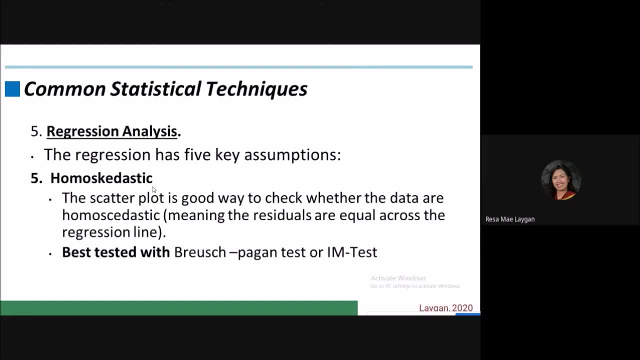 And actually it is somehow related with the normality of the distribution of your data variables in a certain plot. So this can be best tested with bruce pagan test. this is actually a diagnostic test for testing the homoscedasticity and the im test. so actually in homoscedasticity it describes a situation. 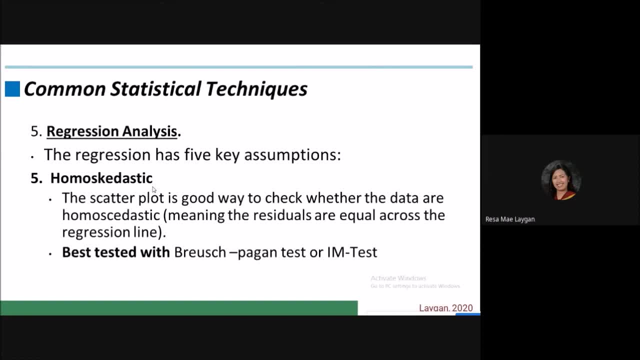 in which the error term or the disturbance of your model, or the random disturbance in the relationship between the independent variables and dependent variable is the same across all world use of the independent variables. so, in order to, in order for the model to be homoscedastic, we 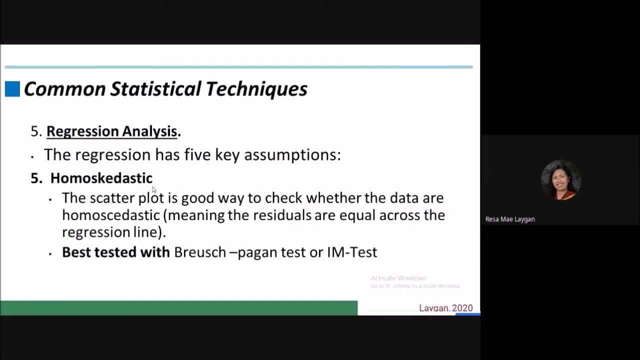 variables. so, in order to, in order for the model to be homoscedastic, we have to address the violation of homoscedasticity, and that is heteroscedasticity. so this happens, the heteroscedasticity is actually differentiated from the homoscedasticity who you can not actually reject there, Theseיע. all and you need no order for the model to be different from the homoscedasticity. but this is what is the size of the error? term differs across values, open, independent variables. so actually there is an impact on violating the assumption of this homoscedasticity because actually 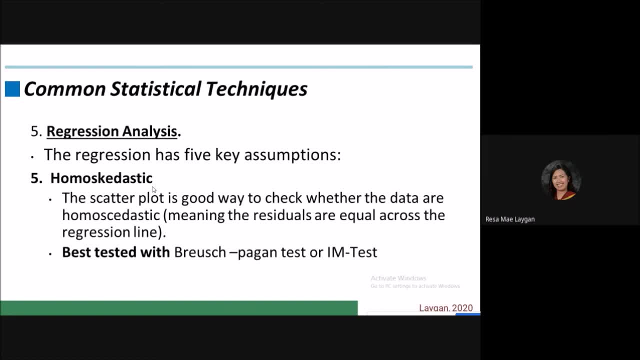 is known, in order for the model to be of the what, the good, or under the goodness, and fit or to improve, you have to follow this assumption. so thus, um some. so that is for the regression analysis. this is only a in an overview. so, under these assumptions, 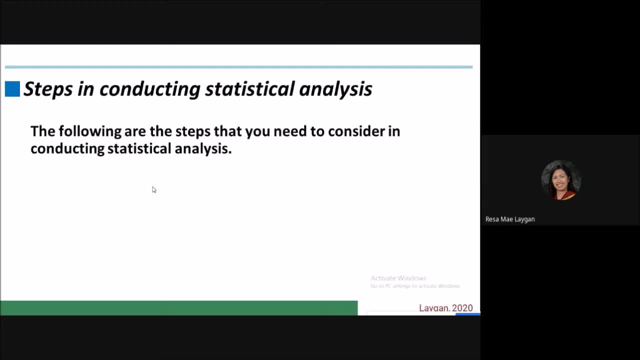 so what are the steps in conducting statistical analysis? so you have to follow these steps and these steps are you need to consider in conducting a statistical analysis. first is you need to identify your research problem, because your research problem will serve as the basis on what statistical technique you are going to use in answering that problem and in analyzing your 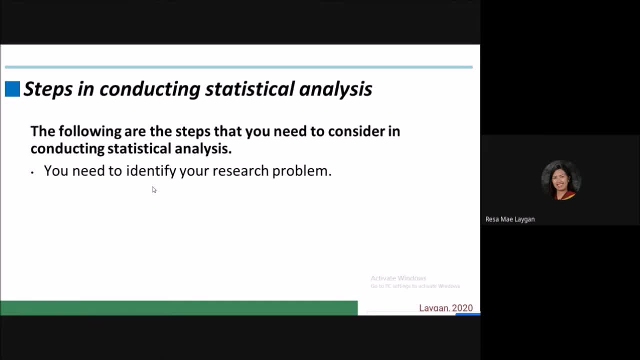 data to come up with a solution or with an answer. and also you describe the nature of the data to be analyzed based on your research problem. so you have to describe if this data is categorical, ordinal or continuous variable, then you may apply the applicable techniques or statistical techniques in describing or in analyzing the data. then you 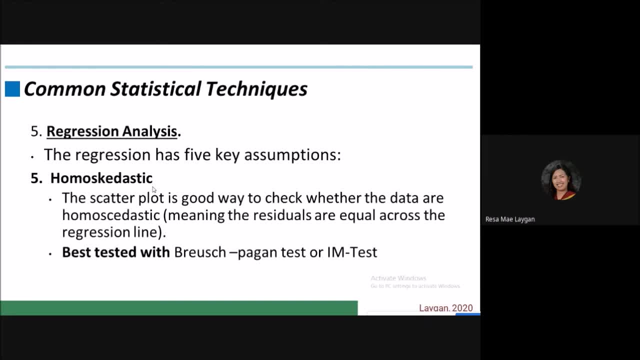 have to address the violation of homoscedasticity, and that is heteroscedasticity. so this happens. the heteroscedasticity is actually different from the homoscedasticity. the heteroscedasticity is present when the size of the error term differs across values of an independent variable. so actually there 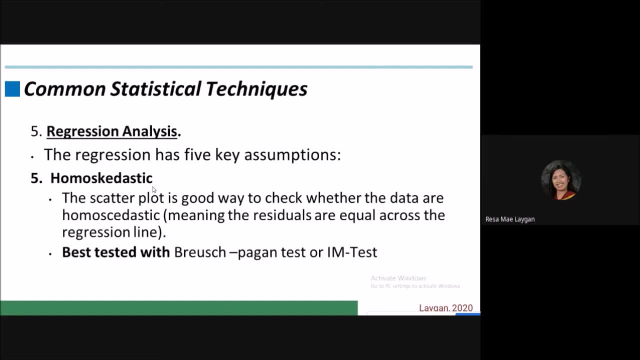 is an impact of violating the assumption of this homoscedasticity, because actually it is the homoscedasticity matters of degree. so you need knowing order for the model to be good, or under the goodness and faith, or improve. you have to follow this assumption. so 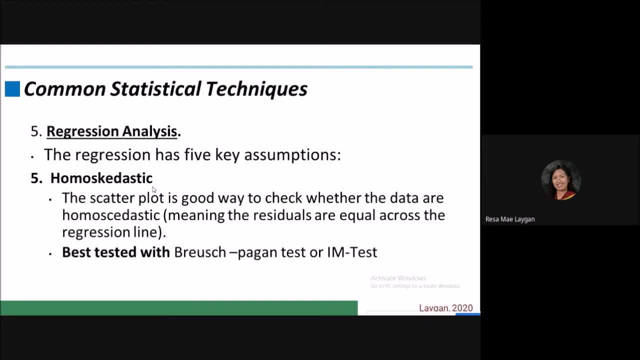 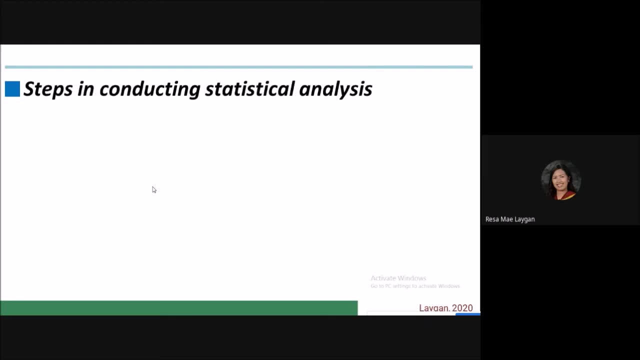 thus some. so that is for the regression analysis. this is only a in an overview. so, under these assumptions, so what are the steps in conducting statistical analysis? so you have to follow this steps and these steps are you need to consider in conducting a statistical analysis. first is 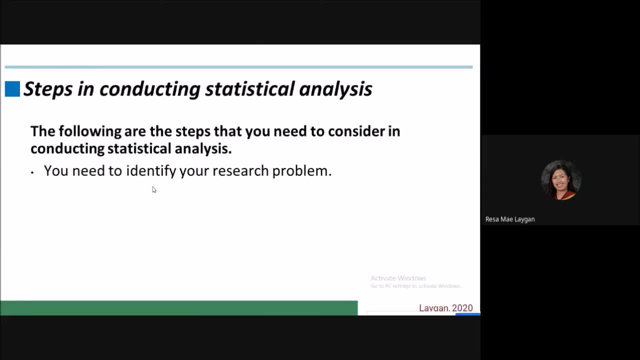 you need to identify your research problem, because your research problem will serve as the basis on what statistical technique you are going to use in answering that problem and in analyzing your data to come up with a solution or with an answer. and also you describe the nature of the data to be analyzed based on your research problem. so you 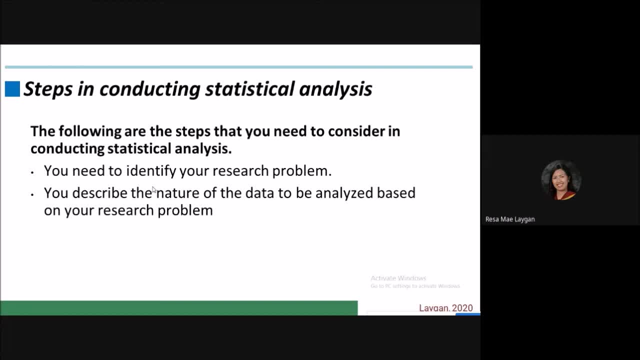 have to describe. if this data is categorical, ordinal or continuous variable, then you may apply the applicable techniques or statistical techniques in describing or in analyzing the data. then you use your research frameworks, especially the empirical model or the equation, to to summarize understanding of how the data relates with each other. 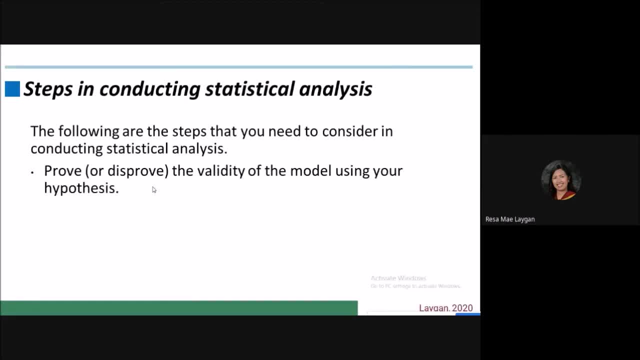 And also you have to prove or disprove the validity of the model using your hypothesis, especially if you deal with inferential statistics or if you are going to test your hypothesis And employ applicable statistical techniques to run scenarios that will help you guide future actions. 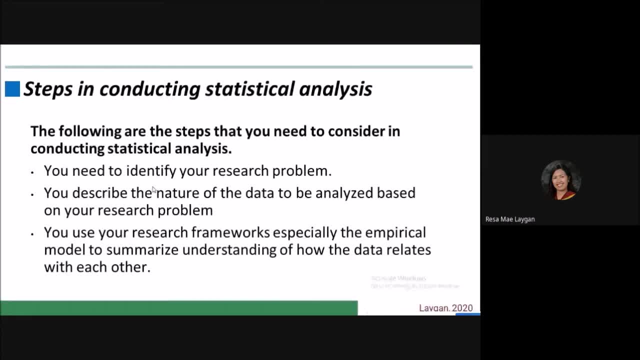 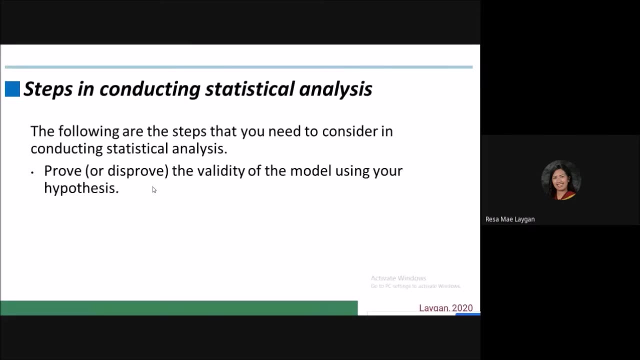 use your research framework, especially the empirical model or the equation, to summarize understanding of how the data relates with each other. and also you have to prove or disprove the validity of the model using your hypothesis, especially if you deal with inferential statistics or if you are going to test. 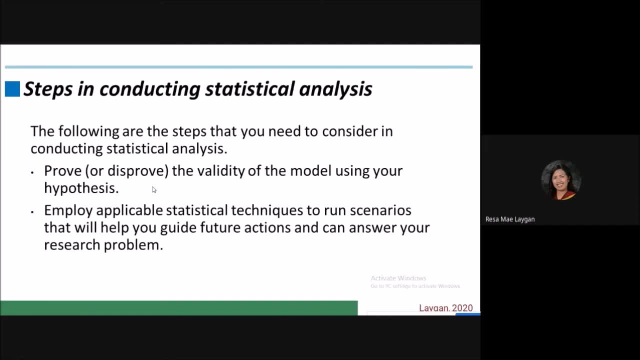 your hypothesis and employ applicable statistical techniques to run scenarios that will help you guide future actions and can answer your questions. research problem. so that is why in each statement of the problem you really have to identify what statistical technique is applicable in drawing an analysis of data from answer. in answering that. 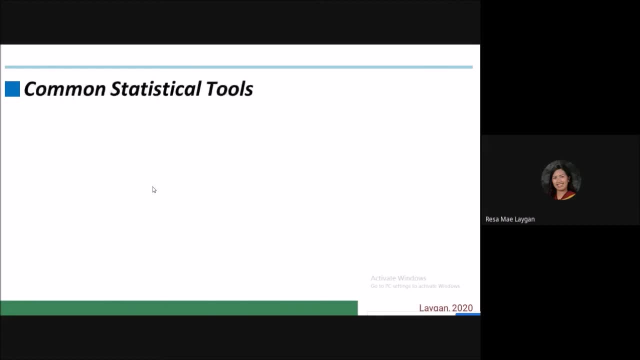 statement of the problem. so, of course, in running or in performing your statistical techniques that you are going to employ, you need this following statistical tools. so you may have this stss. you may download a trial for free from this website if you have money to purchase data. actually, among this two, i prefer stata because it is user friendly. 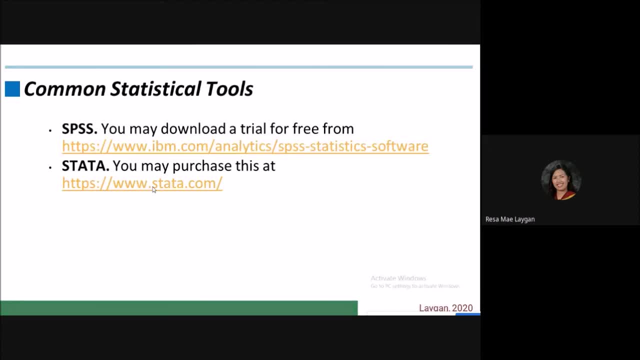 but of course you have to to determine or you have to have enough understanding about the commands of stata. then you may use the megastat. but there are especially in in analyzing the t-test or anova, or you can do also um correlation analysis using the megastat, as long as you know. 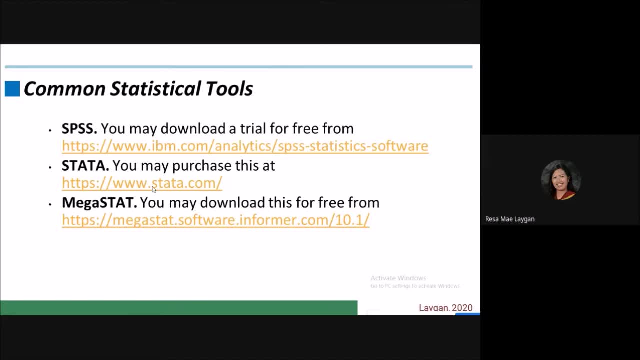 the formulas or the the in on how you input the formulas: in the excel or in the megastat. so, actually, in the excel you need to employ this megastat or you need to gauge this megastat to your excel and we have the r. if you know the codes, if you know how to use the r, 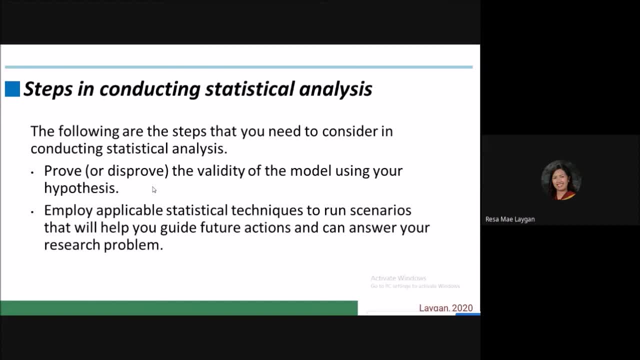 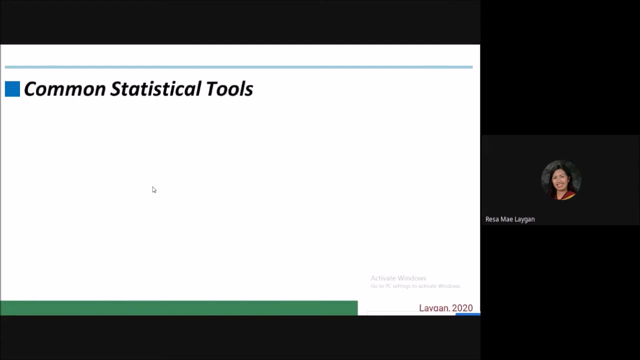 and can answer your research problem. So that is why, in each statement of the problem, you really have to identify what statistical technique is applicable in drawing an analysis of data, in answering that statement of the problem. So, of course, in running or in performing your statistical techniques, 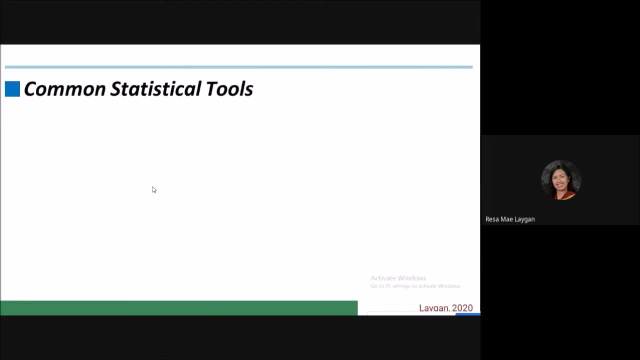 that you are going to employ. you need this following statistical tools. So you may have this SPSS. you may download a trial for free from this website If you have money to purchase data. actually, among these two, I prefer Stata because it is user-friendly. 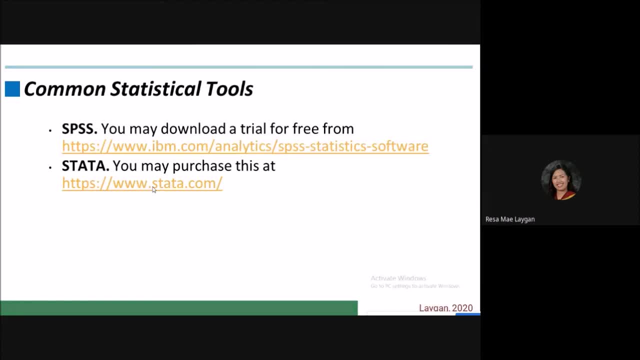 But of course you have to determine, or you have to. If you don't have enough understanding about the commands of Stata, then you may use the Megastat, but there are, especially in analyzing the T-test or ANOVA. 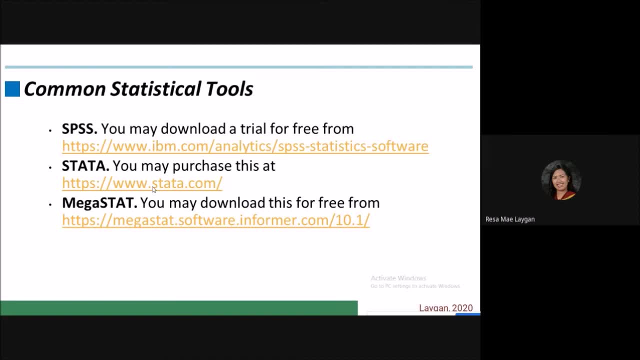 or you can do also correlation analysis using the Megastat, as long as you know the formulas or the the in on how you input the formulas in the Excel or in the Megastat. So actually in the Excel you need to employ this Megastat or you need to gauge this Megastat to your Excel. 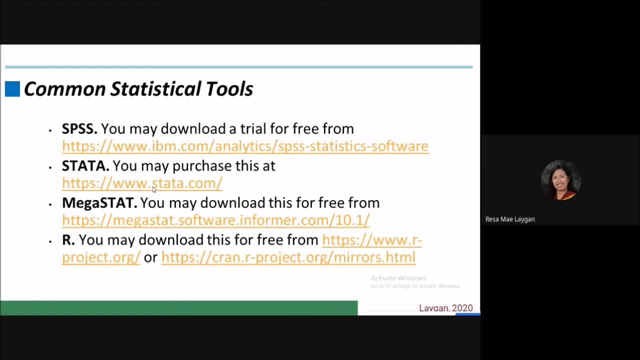 And we have the R. If you know the codes, if you know how to use the R, then you may use R in estimating your data. Actually, you can do regression analysis in R. factoral analysis: Uh, You may use the principal component analysis. 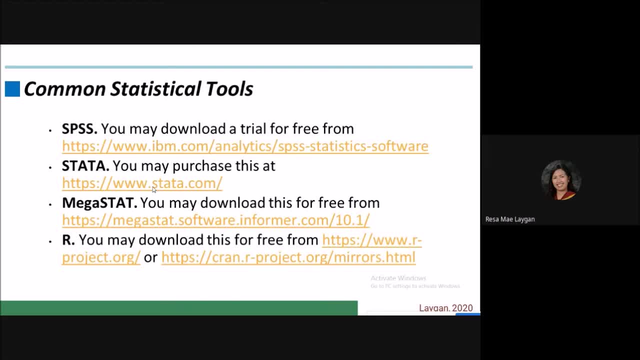 There are different analysis in analyzing your research And those that I presented a while ago. those are the basics, Those are the common statistical techniques And there are lots of statistical techniques that you may use. no Depending on the research problem of your paper.